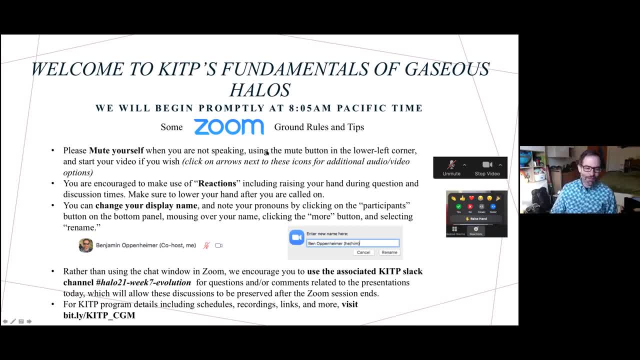 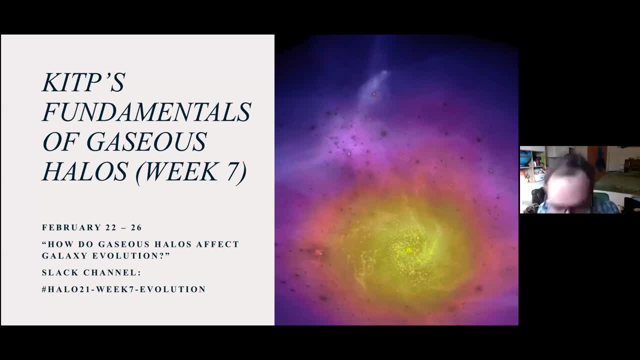 So I'm going to to point out the Halo 21 Week 7 Evolution Slack channel And then I'm going to show our introductory slide for how do gaseous halos affect galaxy evolution. And, inspired by Cameron, I'm going to change the figure here, the visual, each day. So please put your most beautiful and 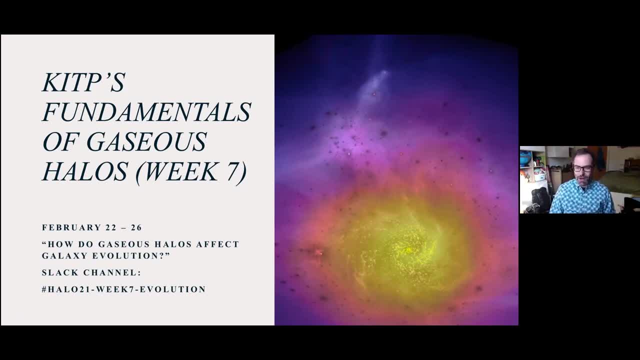 most awe-inspiring visuals from simulations, maybe from observations as well, on the beauty Slack channel, And we'll update this. This is actually a galaxy from one of my simulations that was reimagined in a way showing the cool gas and kind of the brightness level, the hot gas in the colored 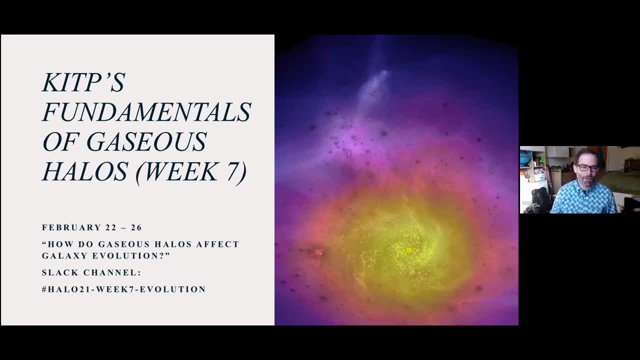 scale, And it also shows dark matter halos, which I think is kind of cool. This is part of a planetarium show that we did here at CU, So I think this is a really interesting question. The you know there's, you know galaxies is a huge field, of course, But to have a galaxy you need 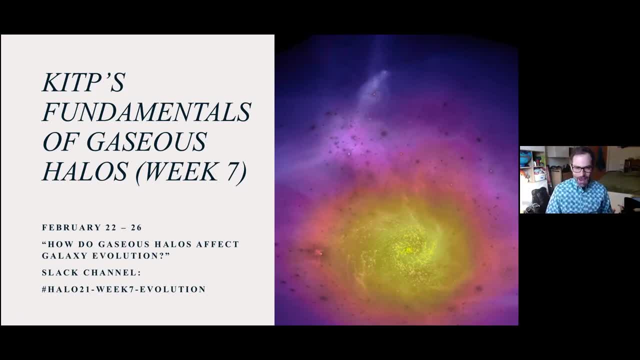 a gaseous component, a gaseous halo, and that comes first. So I like the order of the question: gaseous. how do gaseous halos affect galaxy evolution? Because galaxies need gas to form. of course, We all. 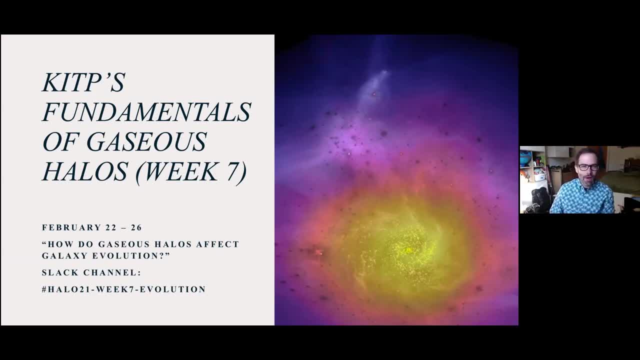 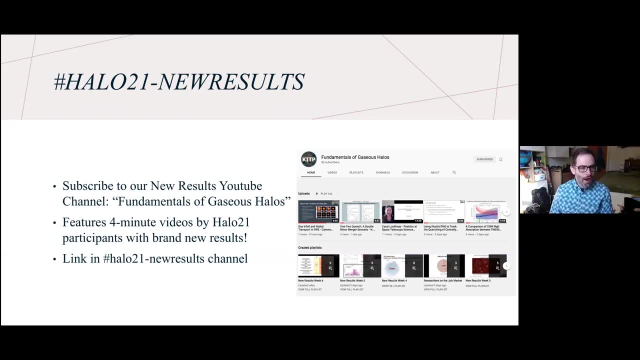 know that, but we will really address that this week. I'm going to go on and go through a few announcements before we get to our featured conversations, As we continue to update the YouTube channel. thanks Cameron for doing all this. we have a lot of new results from last week. 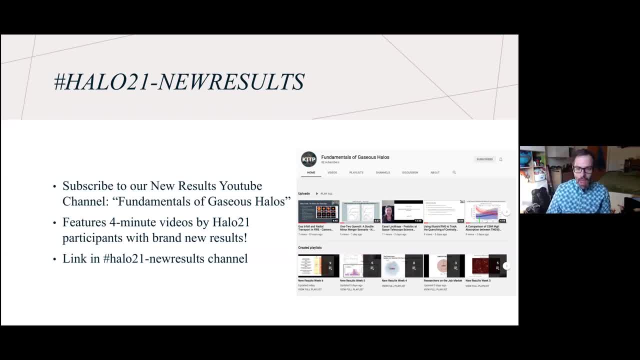 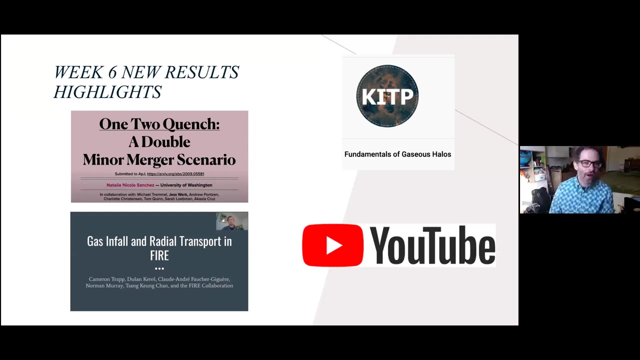 And and Mark gave updates throughout the week And there are nine videos from week six. So this is continuing to get more and more, more and more videos and more each week, especially- And I have, I believe, two to announce, One from Natalie Nicole Sanchez on, you know, showing some nice. 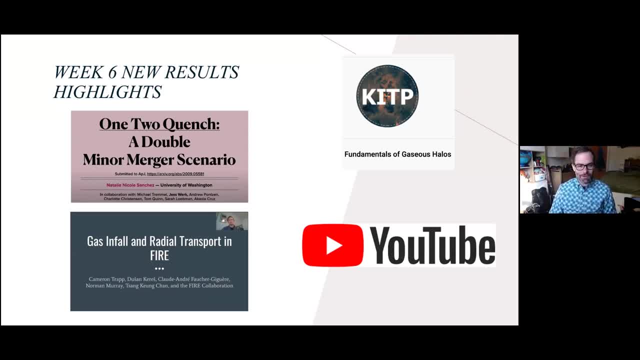 movies actually showing, you know, genetically modified simulations that she has worked on and it's very nice work. And also something that was talked a lot about last week was Cameron Trapp's work on inflows and radial transport in disks. 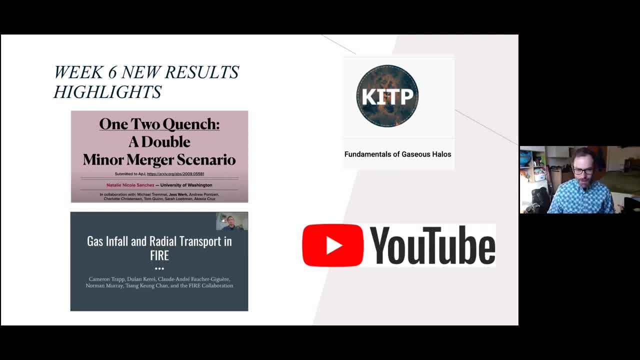 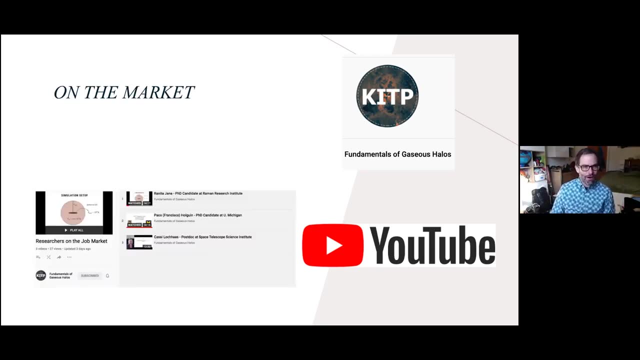 And we saw a lot of these videos last week, So I encourage you to check those out and continue to update those, And we'll post them and announce them throughout the week, And I will also advertise our on-the-market YouTube channel sub-channel on there, And there are three videos on there as well that have been announced. 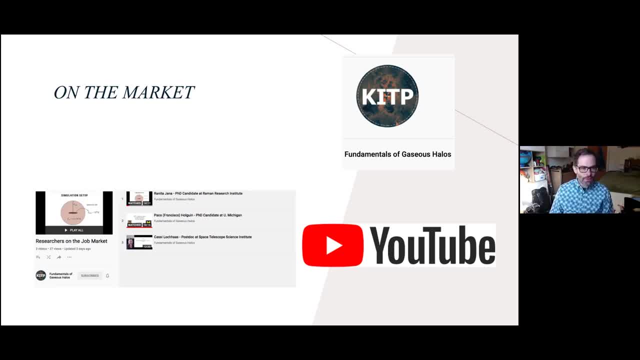 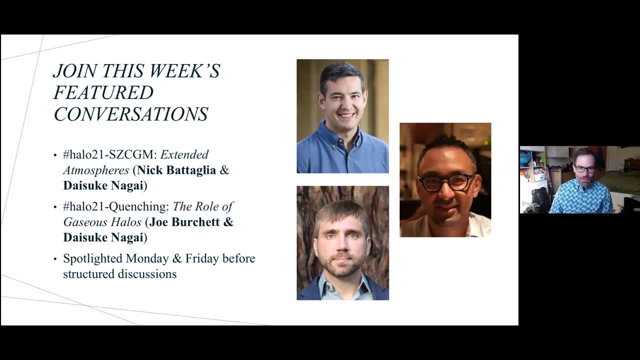 Okay, I'm going to keep on going through announcements and trying to get to our featured conversations this week. So this week we have two And we have Nick Battaglia and Daisuke Nagai talking about Tsunade of Zelda, but CGM and they actually had an after party last week. 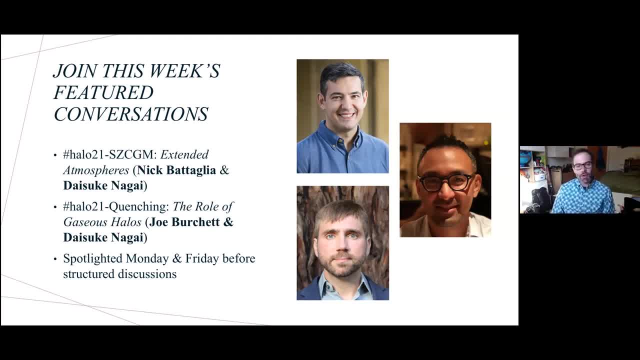 So I will let them talk about their plans and if they plan to do an after party this week. And also we have the continuing ongoing conversation, which is featured this week, of Halo 21 Quenching the role of gaseous halos. 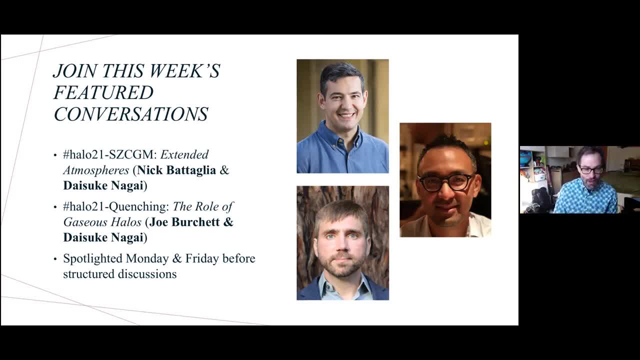 And that's going to be a lot of fun. So thank you so much for watching And I'll see you next week. Bye-bye, So that's a lot of fun. We have two more events led by Joe Burchett and also Daisuke. 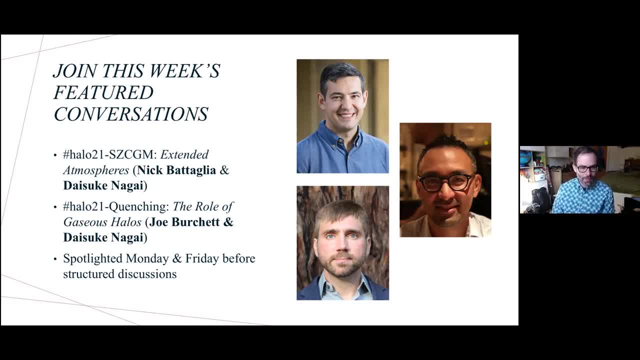 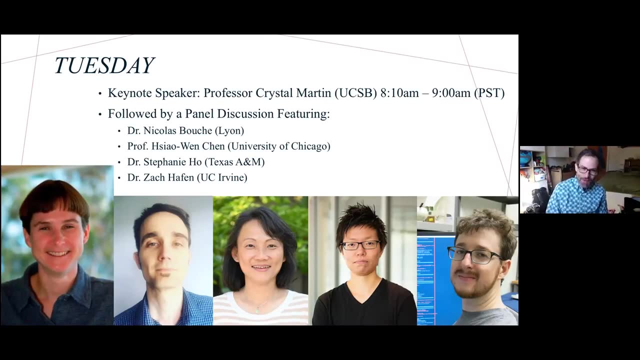 And we will let them decide how to talk about their after you know schedule, their after parties. I believe they have one for Quenching scheduled for tomorrow, So we'll get to that in a little bit, But before we do that- and of course, we have a lot of events today, this week- 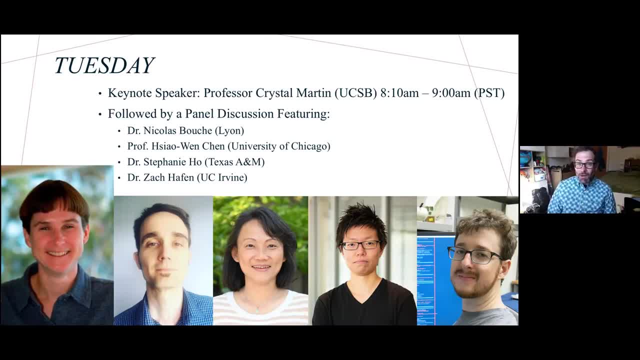 Yes, we have our keynote speaker presentation. It's probably a little bit longer than the first one, But the event is scheduled for Monday, so we will see you there. Bye-bye, Bye-bye, Bye-bye. Professor Crystal Martin, talking tomorrow. 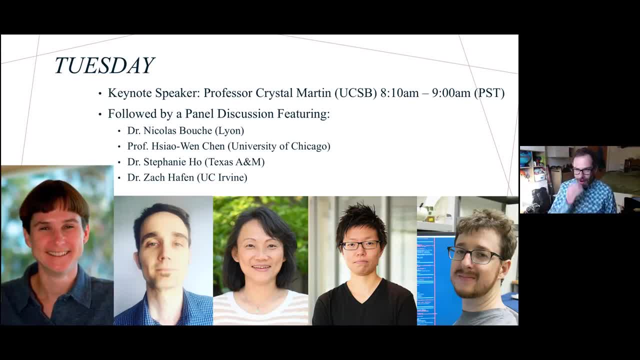 She's a local for KITP And she will give keynote number one with a panel that we carefully assembled with Nicholas Boucher, Xiaowen Chen, Stephanie Ho and Zach Haffin. I reversed those last two names. I don't know the alphabet, but that's okay. 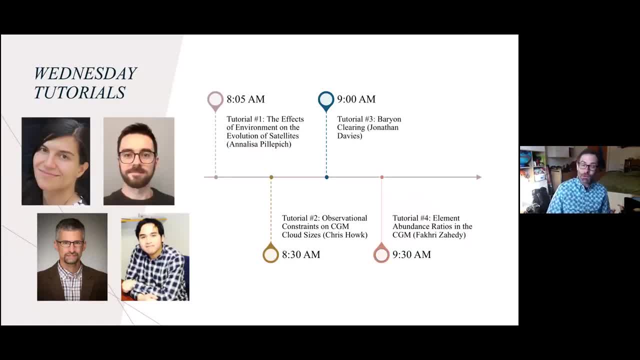 And then on Wednesday we have four tutorials. So it will be very active. I suggest you somehow watch all of them. We'll have the usual breakout sessions. I've ordered them in a way that you know interests kind of are parallel. 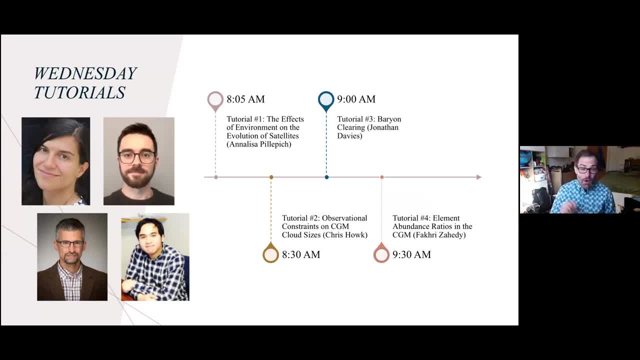 And I think this works for everyone. And if you miss one, if you go to a breakout room, you can go back and watch the recordings of the session that you missed. So we have Annalisa Pilipich talking about the effects of environment. 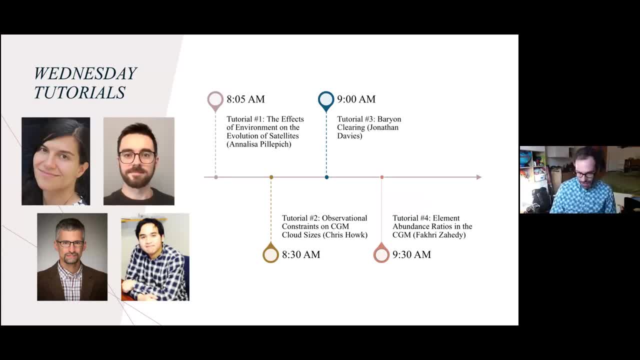 On the evolution of satellites, Something we haven't talked much about but is very relevant for this week. Chris Houck will give a tutorial on the observational constraints on CGM cloud sizes. John Nathan Davis spelled Davies, pronounced Davis. I'm a collaborator, a close collaborator. 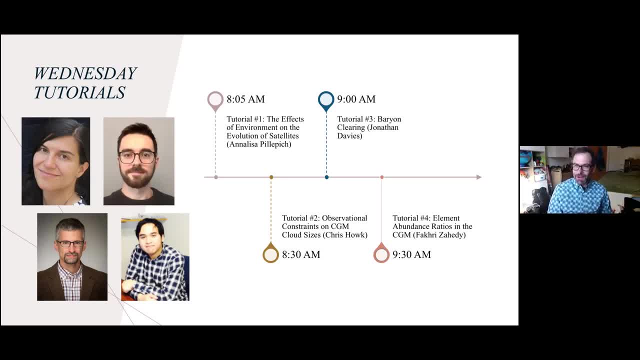 I learned that late to the party. He will talk about baryon clearing, how halos are cleared of baryons- And I think there's a black hole link there, for sure. And Fari Zahedi will talk about element abundance ratios in the CGM and how you can determine them. 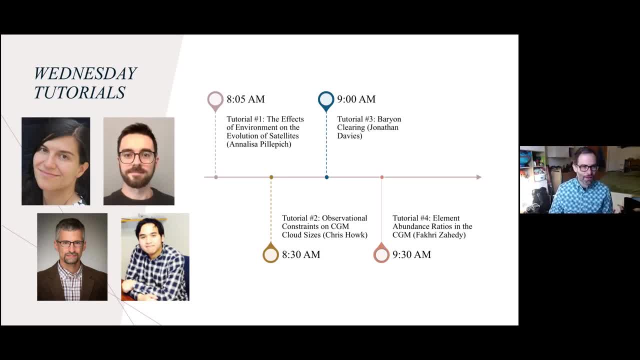 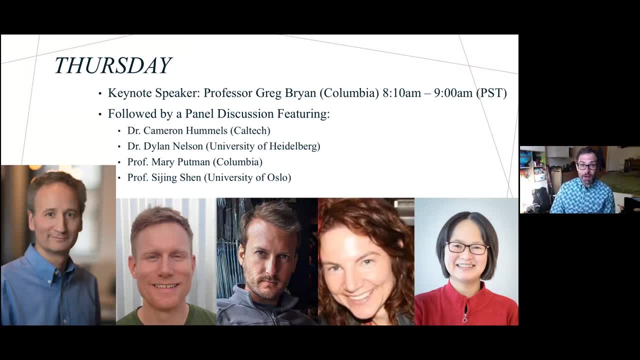 So all very relevant talk tutorials this week. Then Thursday we have our keynote by Professor Greg Bryan, who will talk about more from a simulation and theoretical standpoint, And then we have a keynote by Professor Greg Bryan, who will talk about more from a simulation and theoretical standpoint. 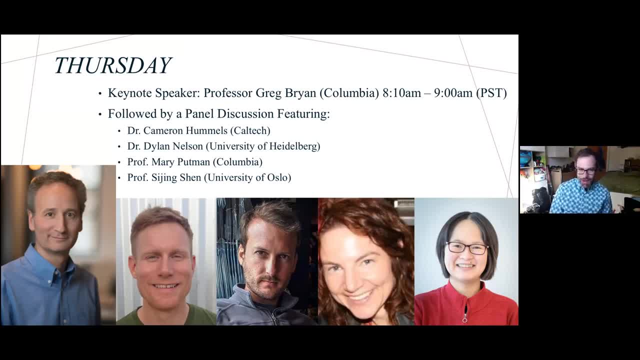 How gaseous halos affect galaxy evolution. And this is another great panel with our co-organizer, Cameron Hummels, Dylan Nelson, Mary Putman, And we got Sijing Shen to join us. She wanted to join us more, but it's late where she is. 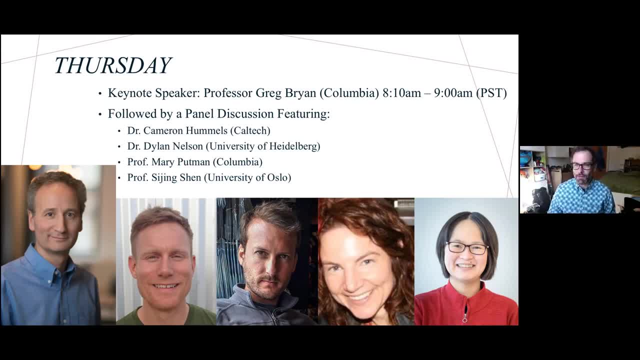 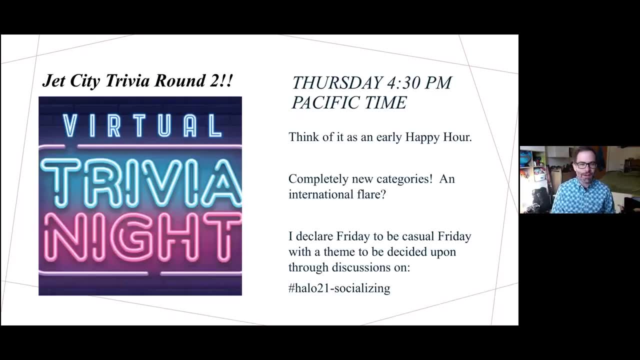 So I'm glad that she will participate in our program this week, Okay, And then on Thursday, Later, Later, Later in the day, we have a social event, Another round of Jet City Trivia. Thanks, Jess, for finding this. 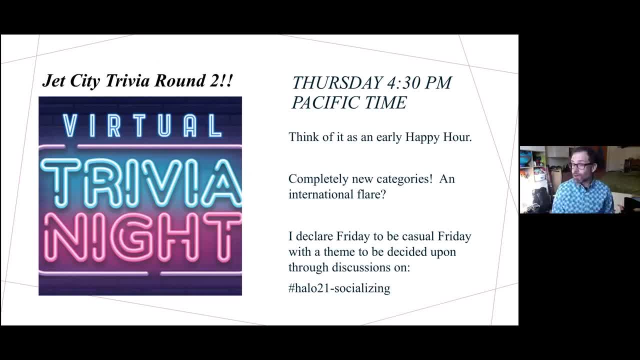 This is great. It's a little bit early And I encourage you to think of it as an early happy hour this week And we will have some new categories. I was pushing for an international flair And you know I think this will be an intense week. 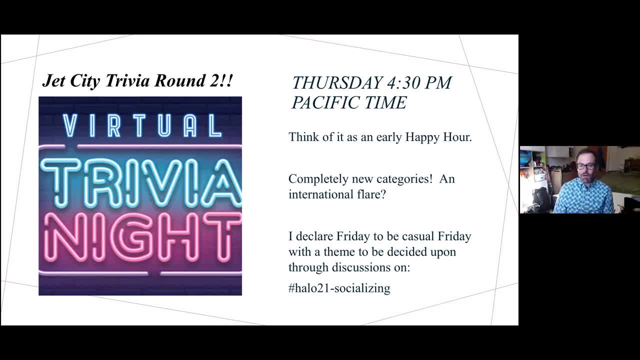 A lot of after parties, A lot, A lot of activities. So I'm going to declare Friday to be casual Friday And maybe we'll have a theme- And you can discuss that- on Halo 21.. I was inspired by Frejka Vanderbort's dressing up and wearing a hat last week. 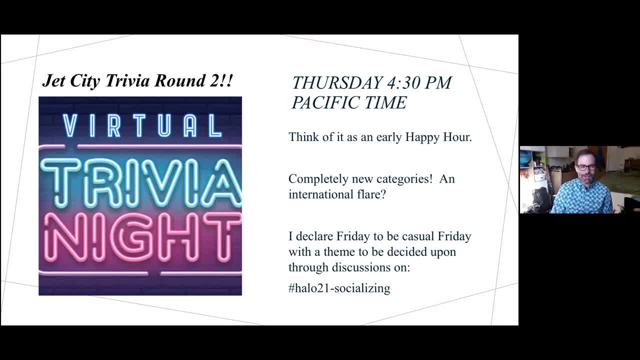 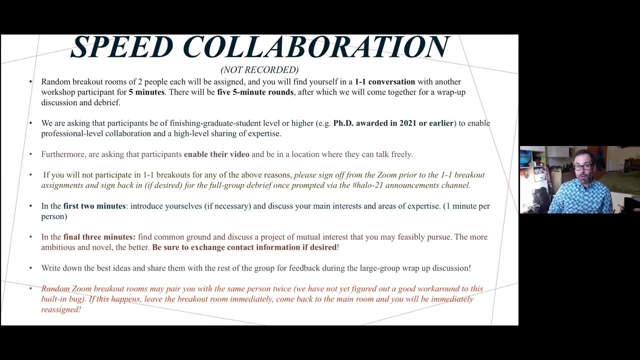 So maybe it will be hats on Friday. So I'm going to take it easy as a moderator on Friday and maybe make it a more informal Friday or more easy. for Friday. We are going to have speed collaboration after our breakout session, So I'm going to have our featured conversationalists prepare to share their slides. 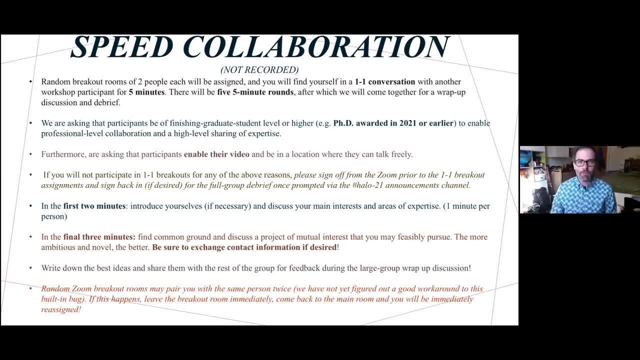 And I believe I don't know who is going first, but I will invite them to speak up And, as usual, we will have these, you know, guidelines for our speed collaboration, So let me see what time it is It's about. 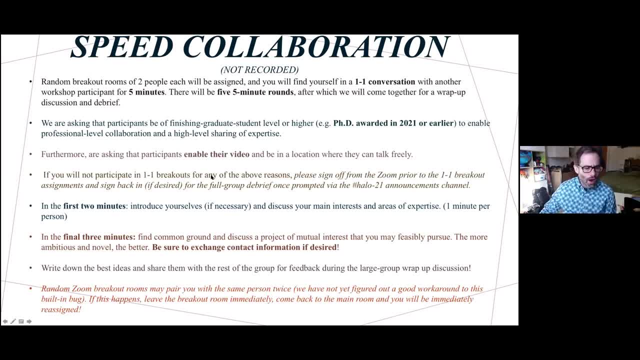 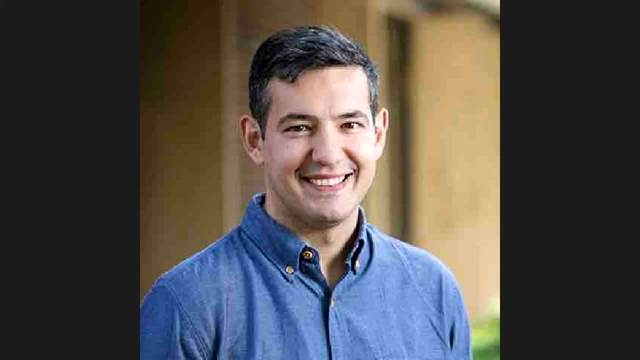 It's about 816.. So if we are ready, are we ready for one of the featured conversations? Yeah, I think Dice UK has a conflict in about 15 minutes, So we should probably go first. Yes, that's why I rushed through it. 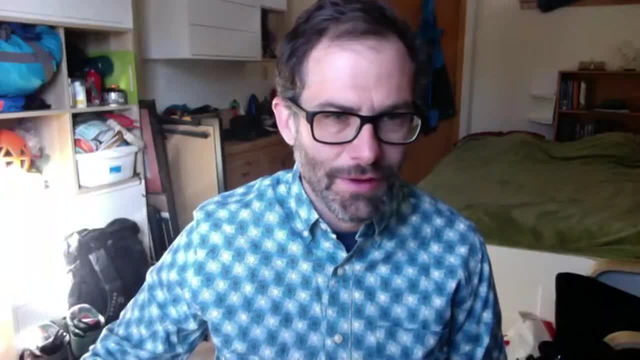 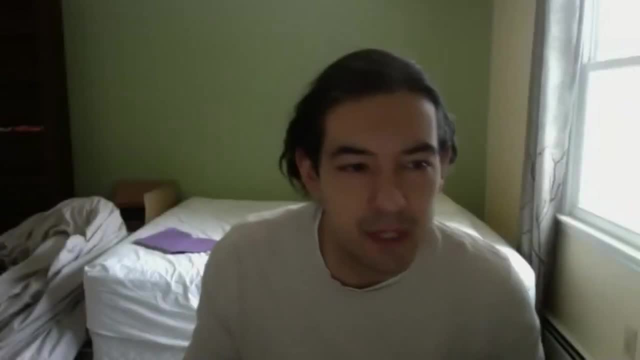 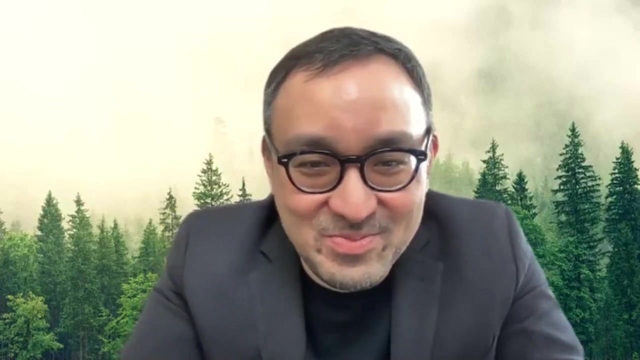 Great, Thank you, Okay. Okay. So, Dice UK, Do you want to share your screen? It's probably best if you share the screen, in case I have to leave. I'd probably, if that's all right, Okay, Okay. 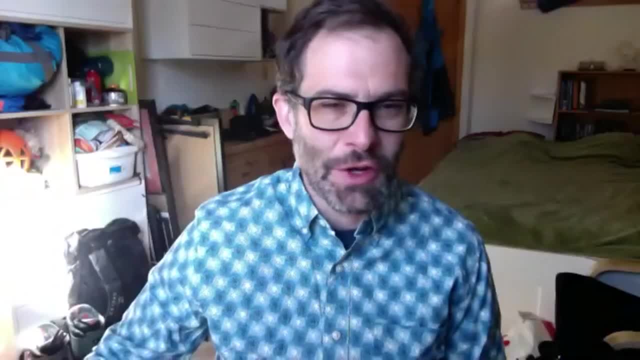 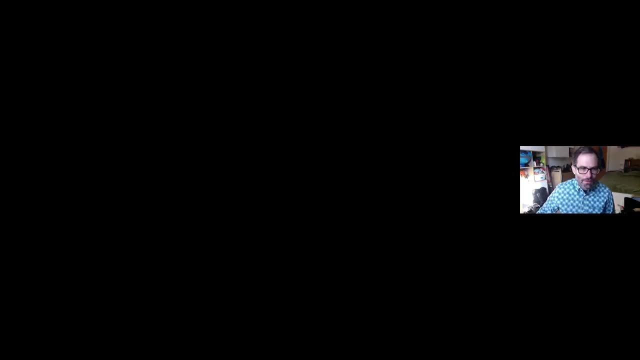 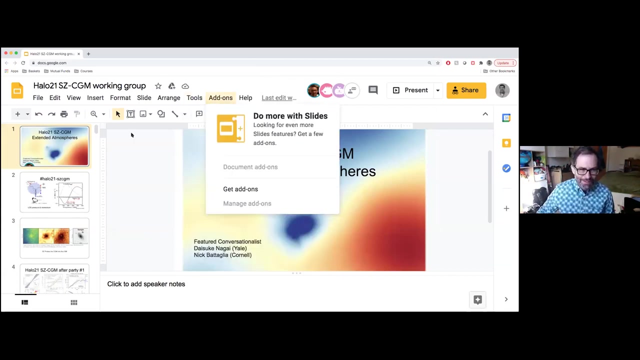 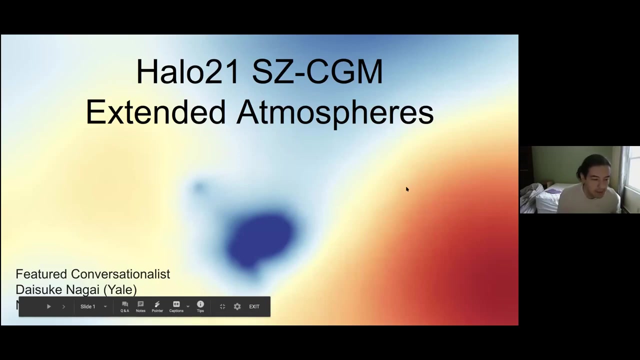 Yeah, Let me just get that ready. I want to make sure you can share the screen. All right, Great, I'll let you go ahead and take over. There's the play Great. So Dice UK and I are the featured conversationalists, as Ben called us for the Halo 21 SC CGM extended. 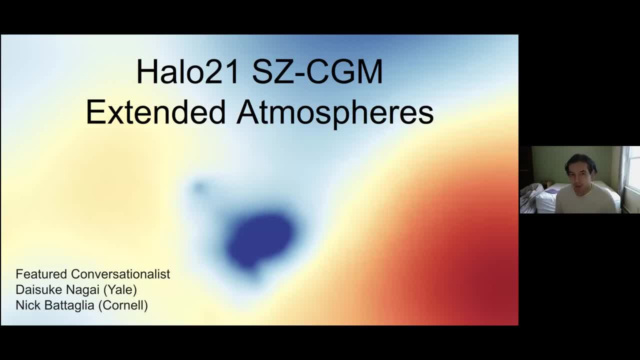 atmospheres discussion this week. So what I thought I'd do was just spend at least two minutes introducing the SC, just for those who aren't familiar, And then we'll go into some of the conversations that we've had already. As Ben mentioned, we had a after party last week that Dice UK arranged. 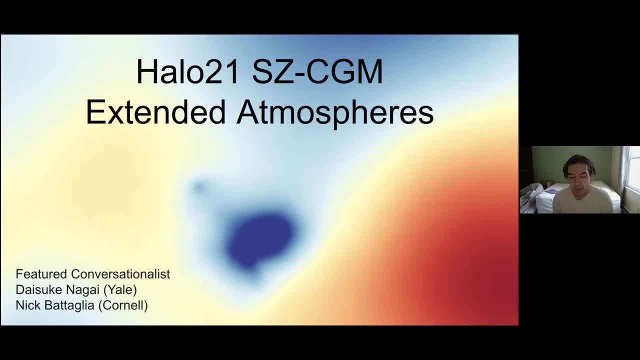 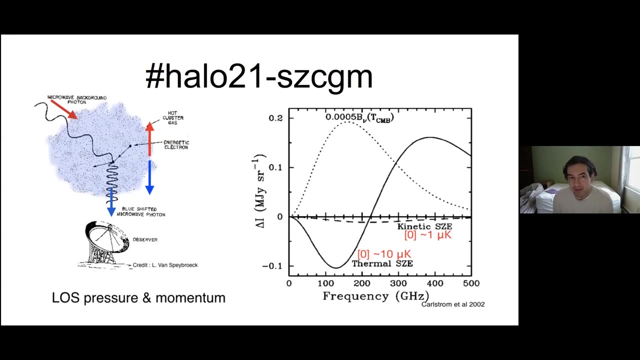 And then Dice UK is going to- if we get there in time- which we should- he's going to outline sort of the questions we want to discuss this week on the Slack channel as well as in the after party Right. So we do have a Slack channel. 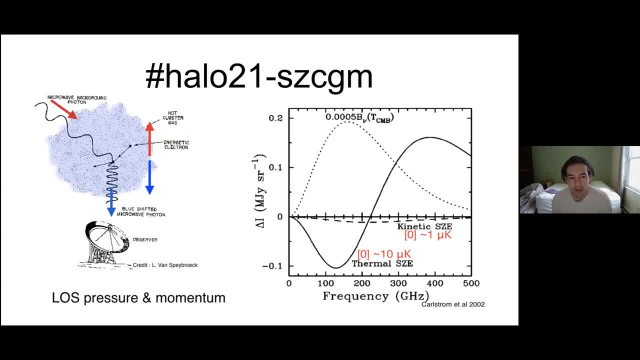 It's been there since almost the first week, I believe, And there we've been discussing various things related to the SC. For those who don't know what the Synergyl-Dolich effect is, well, there's several. There's several Synergyl-Dolich effects. 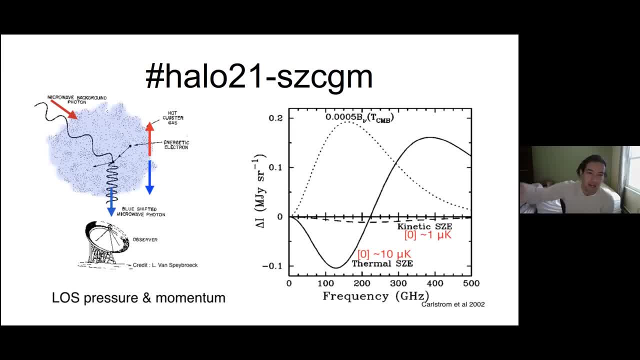 And what it is is we're using the CMB as a backlight And so, as the CMB photons come towards us, right, they interact with free electrons along their journey to us And some of the ways they interact. well, there's one effect where some CMB photons 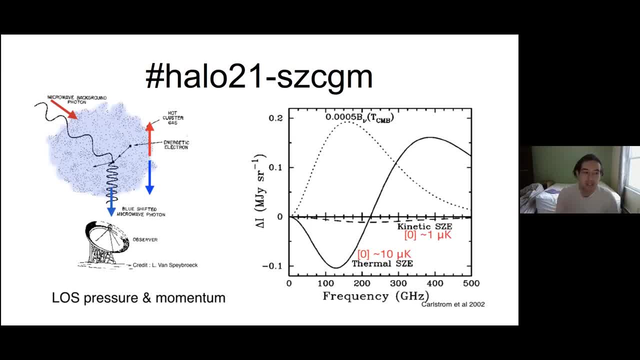 inverse Compton upscatter off hot free electrons. That's called the thermal Synergyl-Dolich effect. That's the more, I guess, familiar SC effect. It was detected way back In the 80s and that's the amplitude of that effect is proportional to the line of 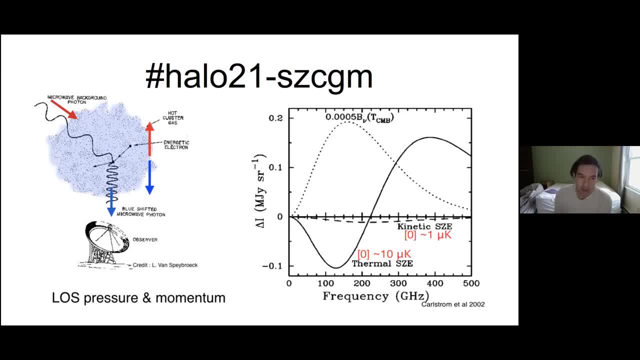 sight electron pressure, which can also be interpreted as the integrated, integrated thermal pressure along the line of sight, which can also then turn into the thermal energy. Then there's the kinematic or kinetic SC effect, and this is the fact that free electrons have a peculiar velocity with respect to the CMB. 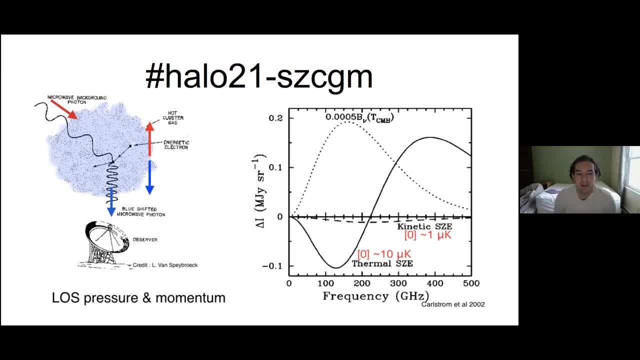 So they act like A moving mirror and that gives the CMB a Doppler boost. right, So this looks. everybody's familiar with the Doppler effect. So if the free electrons happen to be moving towards us, that's a blue shift. 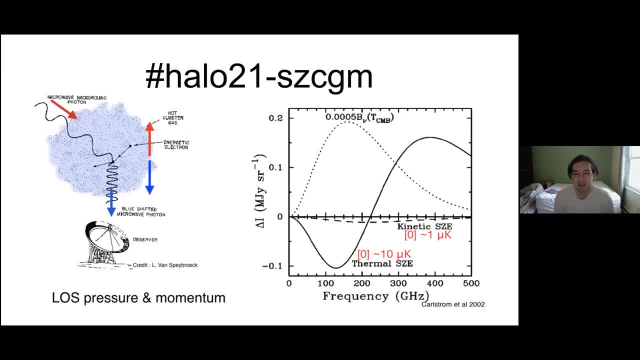 If they're moving away from us, that's a red shift and that's a slight change in the CMB temperature. So these two combined effects right. we have line of sight pressure, line of sight momentum. If you're able to split apart the momentum and have some estimator for the velocity of 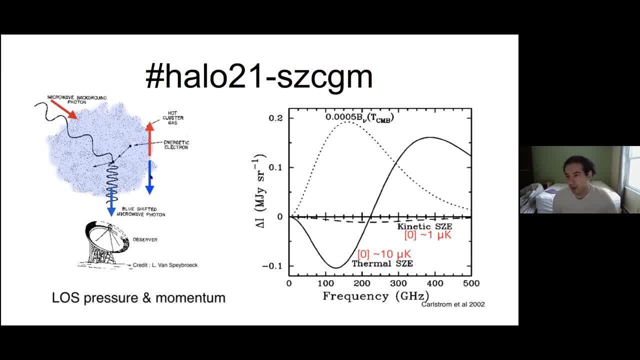 those electrons. then you have a measurement of the pressure and you have a measurement of the density. Therefore, you have full thermodynamic information on these systems. What's really neat is one: the kinetic SC looks identical, at least the first order to the 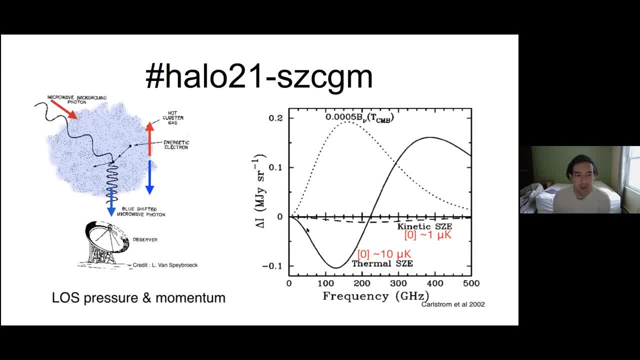 cosmic microwave background, So it just looks like a black body with a slightly different temperature. And the thermal SC actually has this unique spectral distortion where you have a deficit of photons at low energy and excess at high energy. Okay, And this is. this shape right here is unique to the 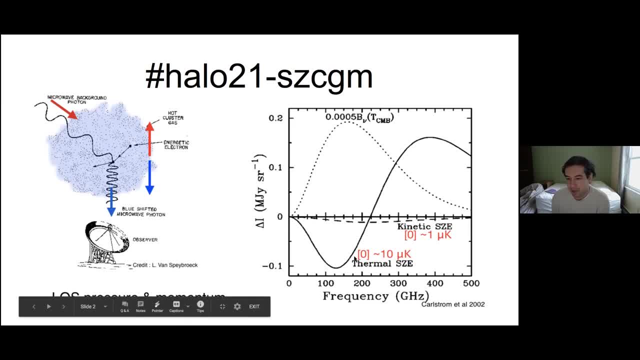 So if you measure your CMB in various different bands, which we do, you can in principle separate out this particular thermal SC signal from the other signals like dust, like the CMB, like radio galaxies. So this is what we're doing. 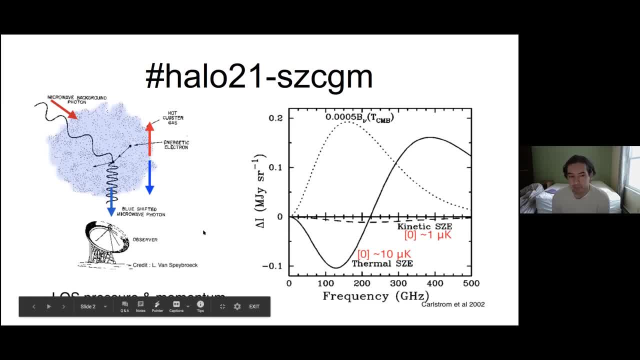 These effects are particularly small. We have measured individual thermal and kinetic SC effects in galaxy clusters. But if you go down to sort of the massive galaxies to just regular galaxy scales, you tend to have to stack or cross correlate to pull out these signals as they are, you know. 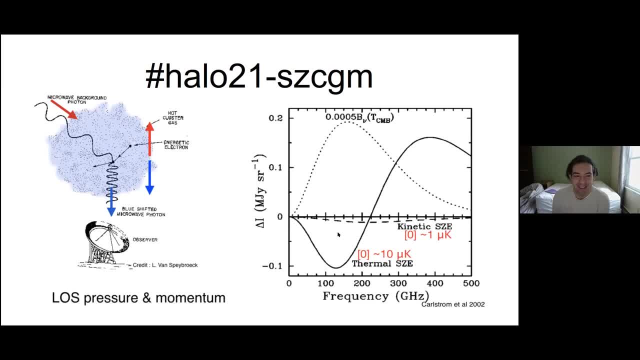 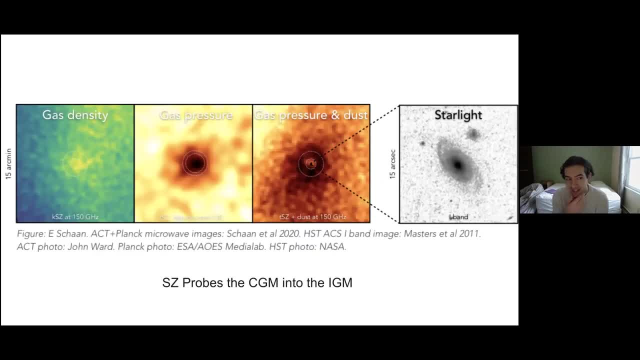 at least several orders of magnitude smaller than the, than the fluctuations in the cosmic microwave background, And these are extended. What's really nice about the SC is that you're not really sent Well. it's a pro and a con right principle. You really want to get down in there and measure the, the thermodynamic properties inside. 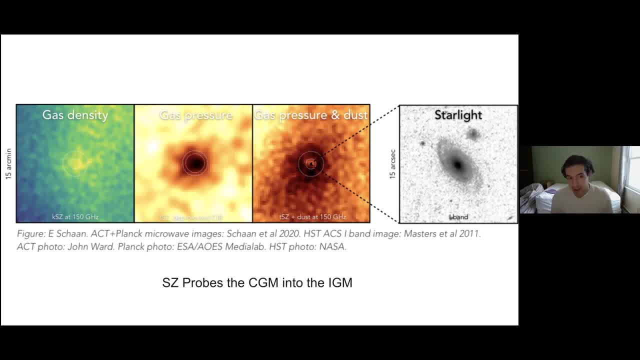 The galaxies and that you in principle can do with local galaxies, or if we have really really large telescopes but we're really diffraction limited here. So at least with the current ground based experiments we have about a resolution of one. 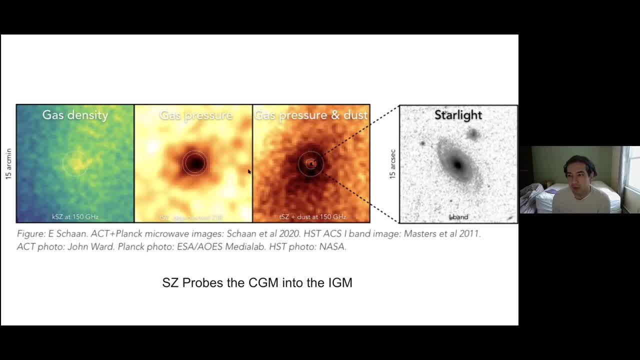 arc minute, but we can probe all the way up to several virial radii so we can measure basically the transition of the IGM to the CGM, which is really nice in both density and pressure. So just to give you an idea, that's why we're calling it extended atmospheres, right? 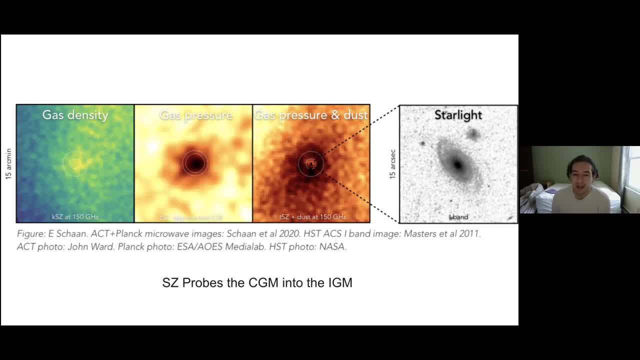 Where you know here's. here's a galaxy over here and it's at the very, very center. also potentially has some dust in it, But you can see. we measure the thermal velocity well beyond where the extent of the stars in the galaxies. 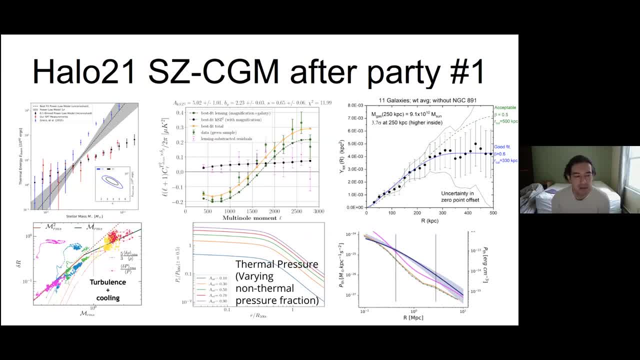 So we had a discussion last week- I'll let Daisuke mention this a little bit more- And there were several recent results that people presented on both the kinetic and the thermal SZ. We also had some talks about some theoretical modeling, the various models people have. 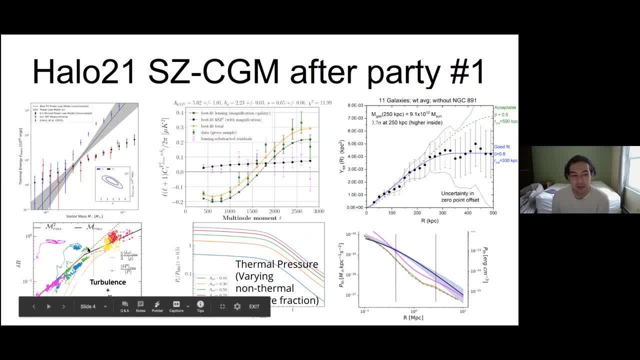 and as well as inferring properties of turbulence from the thermal SZ. So if you can measure the pressure fluctuations, you can infer something about the turbulence in the CGM, which is really cool, And people have done this for the intercluster medium. 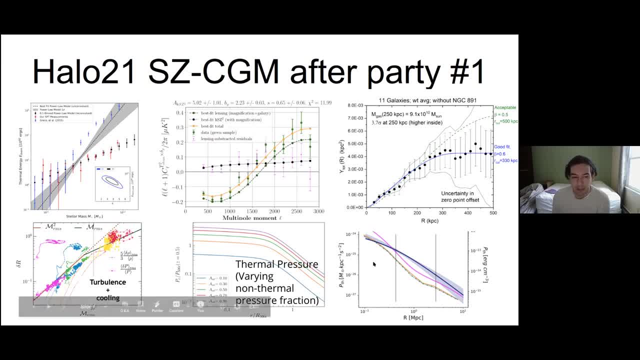 So these are all there. There's a video that Daisuke posted on the Slack channel So you can all go. if you missed it, You can go watch that. You can watch the video and watch some of the discussion as well as the slides are. 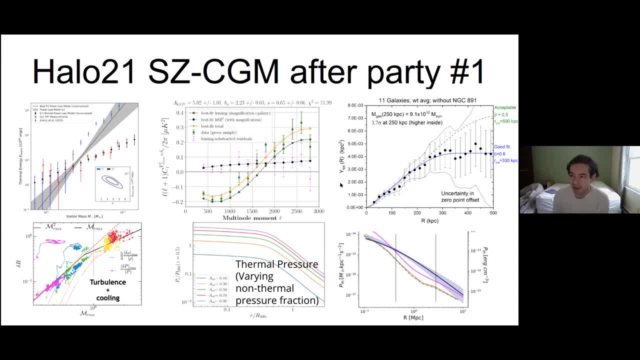 linked actually to this slide deck. So once Daisuke and I are done talking, if you just continue on down on the slide deck, you can see all the slides from that after party we had last week. So with that I'm going to pass it off to Daisuke, who's going to tell us about what. 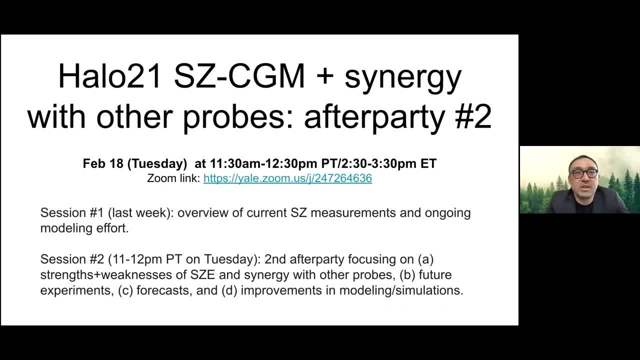 we want to talk about this week. Daisuke Ito, Great. Thank you, Nick. So we'll follow up on the conversations that we started as a part of the kickoff After party last week. we're going to have a second one on tomorrow. 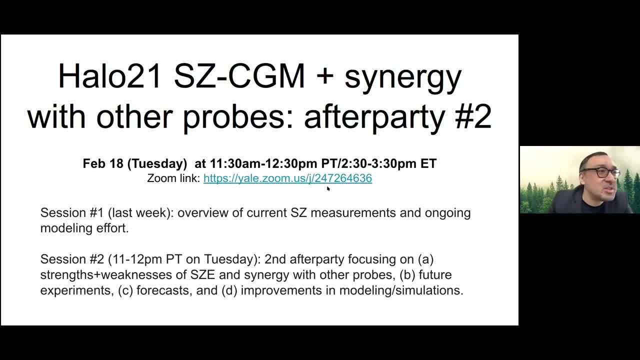 It says 2018, but it should be corrected to 23rd at 1130 am to 1230 pm on the Pacific time, 230 to 330 on Eastern time. So here's a Zoom link And the last week we talked we had a brief overview of current SD measurements and ongoing. 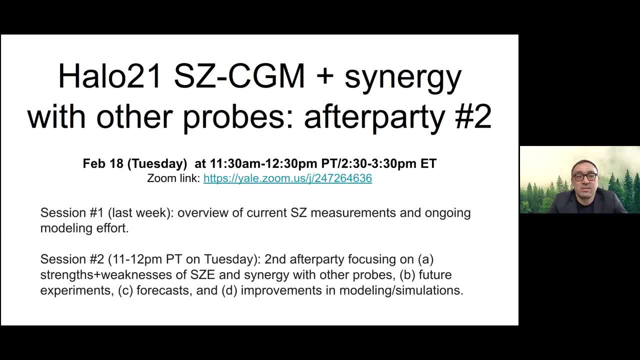 modeling effort. So in the second after party We are planning to dig a little bit more, dig our teeth into some of these topics, discuss further about strengths and weaknesses of the SZ technique, possible synergy with other probes. We want to discuss also about the future experiments, what kind of science that can be enabled by. 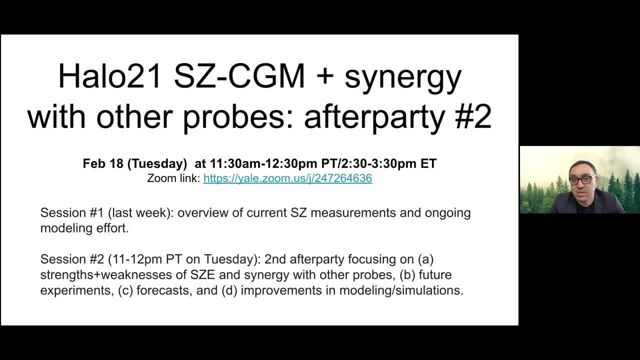 using SZ effect in combination with some other multi wavelengths probes. We also want to start discussing more about how to make a specific forecast for different surveys, different techniques And some of the improvements in theoretical and computational modeling that needs to be done in order to develop the science case. 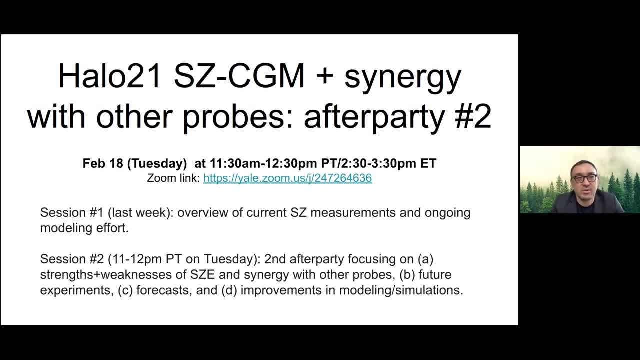 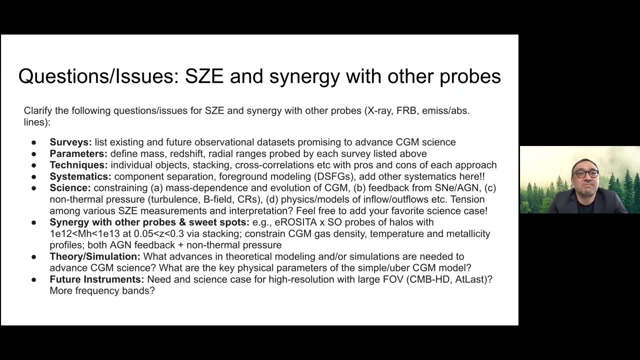 So that's going to be the main focus of the topic for the coming week. for tomorrow And there are a number of typos. Instead of 11 to 12, I will correct this 1130 to 1230 tomorrow. Can you go to the next slide please? 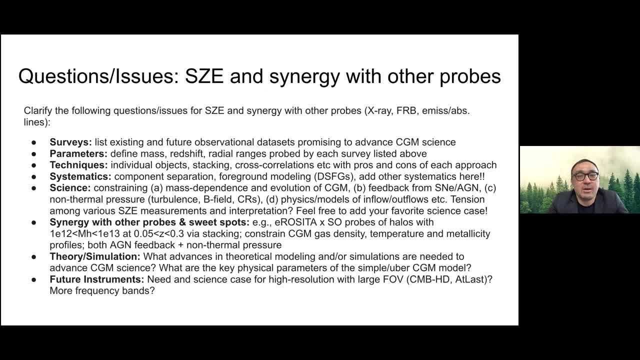 Okay, All right, All right. the questions and issues that we plan to discuss at the after party tomorrow- This is similar and analogous- is in part motivated by our conversations for the future observations that's coming up in the following week, So last Friday. 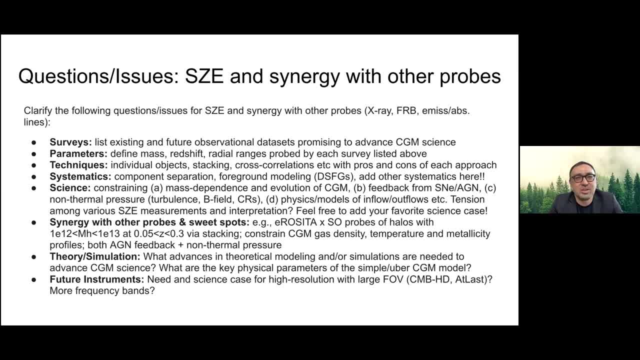 we talked a little bit about. what are some of the questions that we would like to address and discuss in order to define the science case that could be enabled with future survey. What are some of the parameters, like mass redshift and radio range, that are? 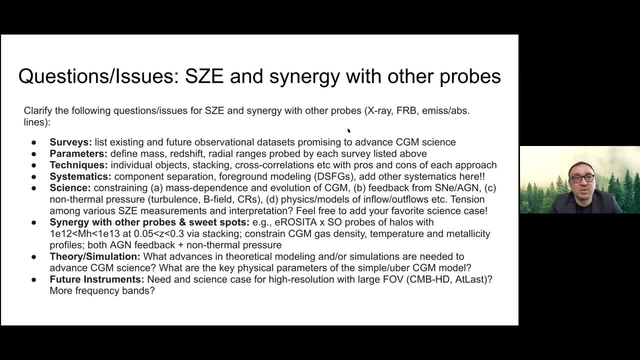 probed by different techniques and surveys. We also want to talk about various ways of detecting SZ effect, such as the detailed studies of individual objects to stacking and cross-correlation techniques. What are the pros and cons of these different approaches? In the process, we talked about a number of systematic uncertainty facing SZ measurements. 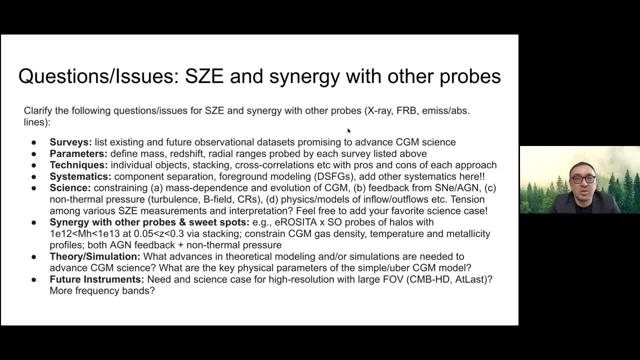 some of which has to do with how to do component separation. There are multiple sources in microwave sky that needs to be separated and distinguished using multi-frequency observations, so how well can we actually do that? We need to think about how to do forward modeling and 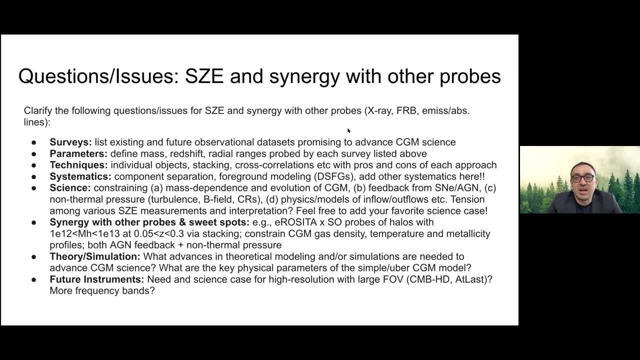 things like dusty star forming galaxies are extremely bright and therefore there are the potential contaminants for many of the techniques. We also want to discuss how to mitigate these systematic uncertainties and how we would want to discuss those systematic uncertainty that we are expecting to get in the coming years. 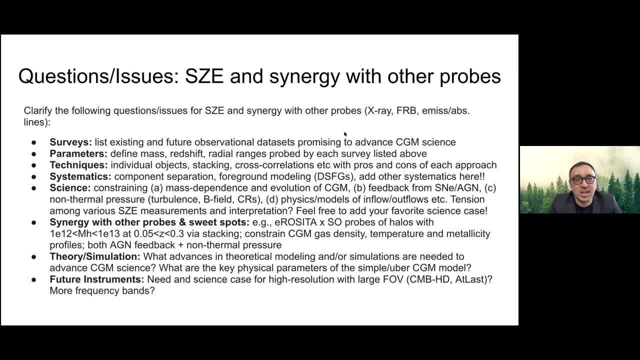 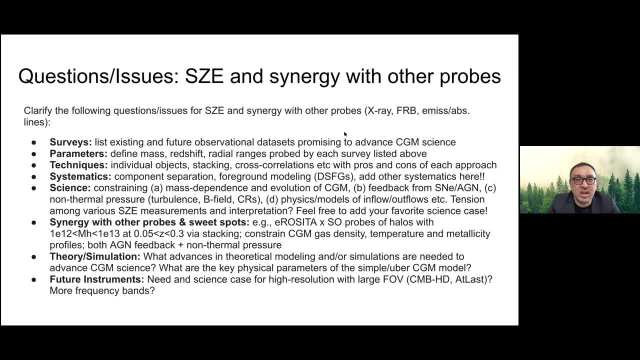 Bye, bye, SZ effect and, of course, how we can actually combine SZ effect with other wavelengths. and what are some of the sweet spots in terms of halo, mass, redshift range and radio range that can be enabled by combining SZ effect with other probes. 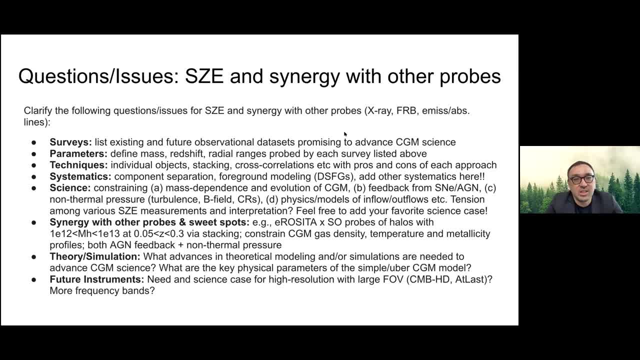 We would also, then, want to discuss about the theoretical challenges and also simulation that are needed in order to refine the predictions, and also think about the simple and possibly Uber CGM model that can be used to interpret multi-wavelength observation as well as making forecasts for future surveys. 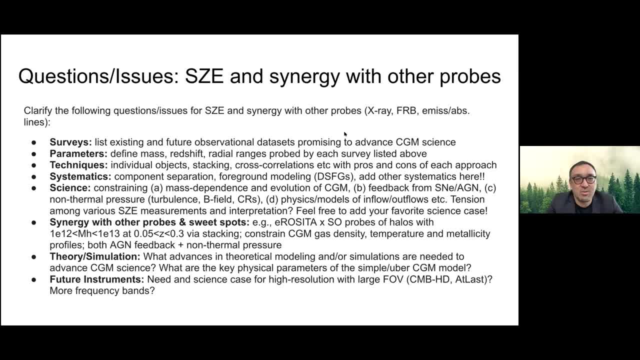 And then, last but not least, we would then want to think about whether we actually need new instruments such as high-resolution SZ, spatial spectral imaging capabilities with large field of view, such as CMDHD, ATLAS. These are proposed missions. These are proposed missions that are under consideration for future ground-based telescopes. 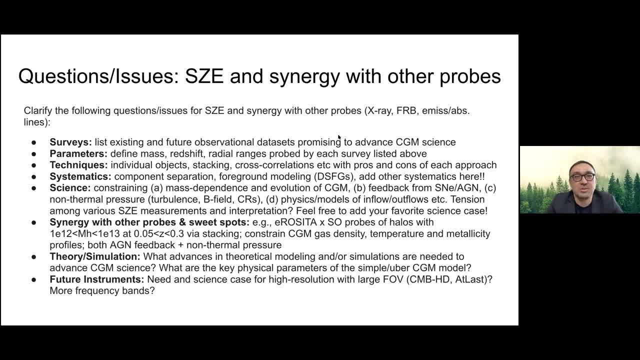 and how many frequency bands are needed in order to mitigate all of these systematic uncertainties. So we have loaded questions We know we just had. from the first after party we got a glimpse of where we are now, but there are so much more we could do over the next few years, to decades to come. 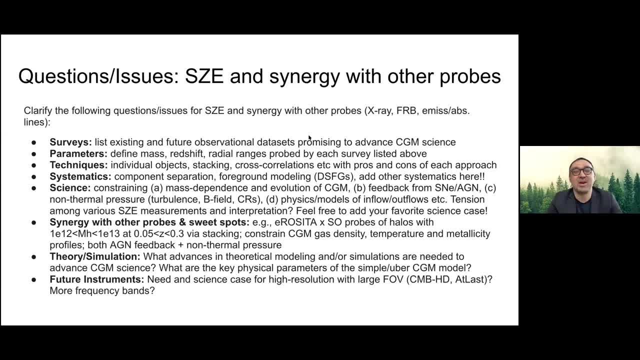 So we'd like to unpack some of these questions and we'll think about how best to organize in order to To come up with some specific idea on directions and possible project that we can actually pursue together as a part of the Halo 21 workshop. 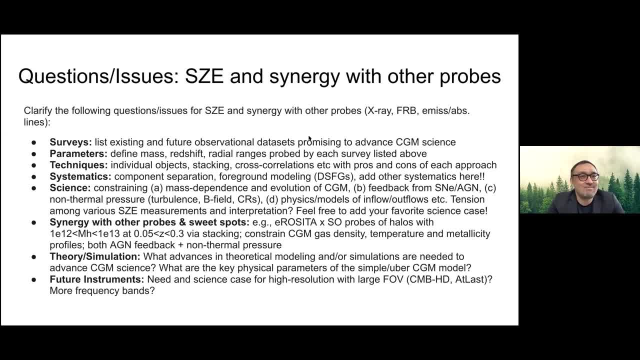 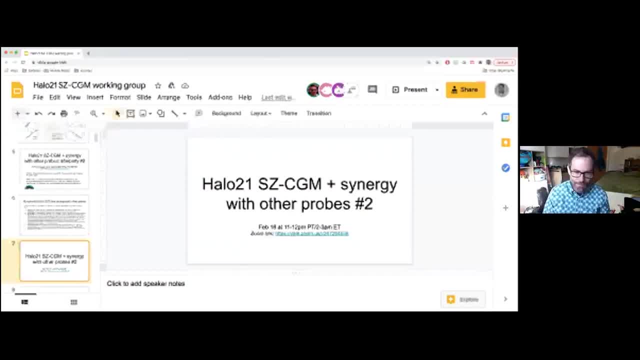 So I'll stop here, Okay, Thank you. Thank you, Daisuke, Thanks for doing that And you're like up against. I think you have to teach like on the half hour, So you have a few minutes to spare. 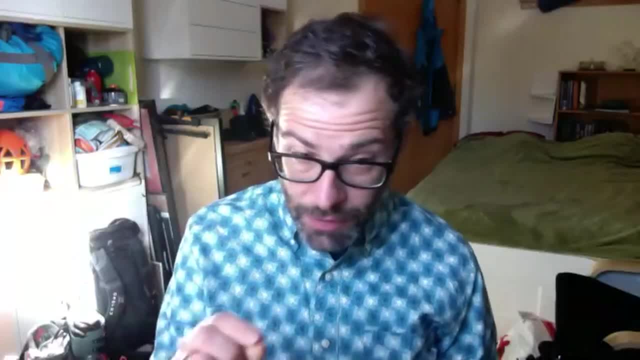 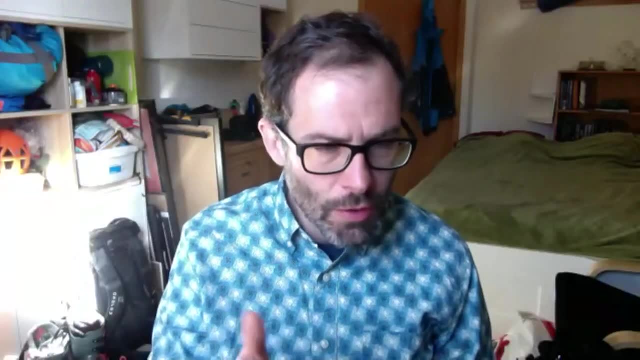 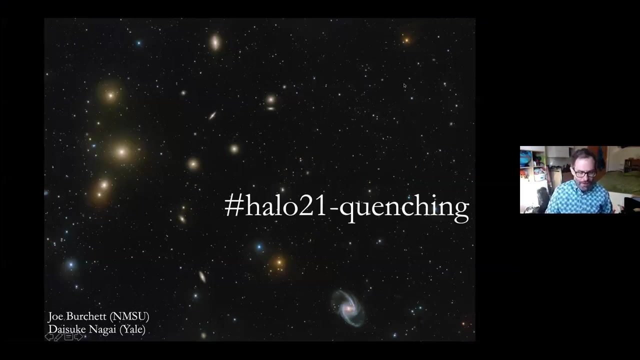 Great job And I believe you're involved with Joe in the next after party, So I am going to Turn it over. I think Joe is going to talk now and I think we are going to have two concurrent after part- or no, not concurrent- two consecutive after parties tomorrow. 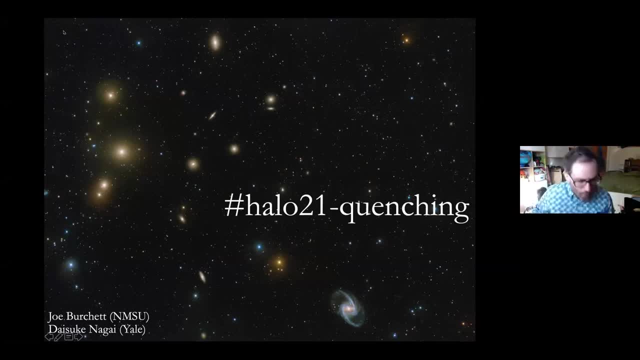 And Joe will confirm or deny that rumor. Yeah, And hopefully you can see my first slide here. Hello, Well, you're good. Okay, Go for Joe, All right. So yeah, I'm here this morning to introduce our conversation group, Halo 21 Quenching. 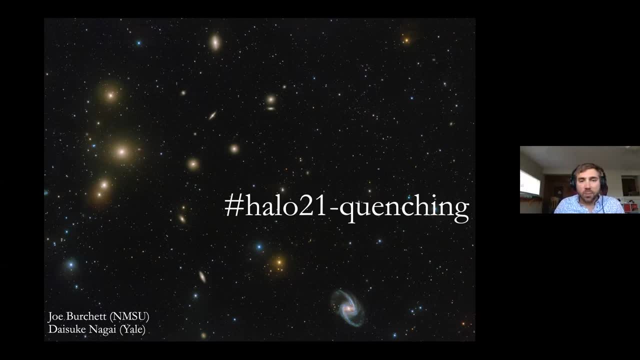 So this in the background here is a breathtaking image to me, an image of the Fornax cluster, which is very much not what you might visualize for the prototypical galaxy cluster, But I think Daisuke had this kind of environment in mind. 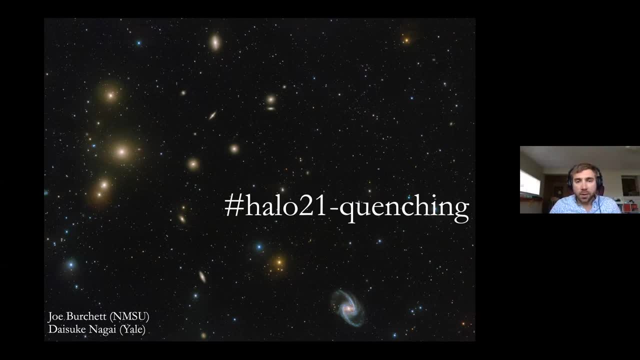 Whenever We sort of conceived this, this conversation group, and and we did so with a subtext of galaxy quenching and massive halos and the cosmic web. So the Fornax cluster is is very much a dynamic environment that is in an active state of. 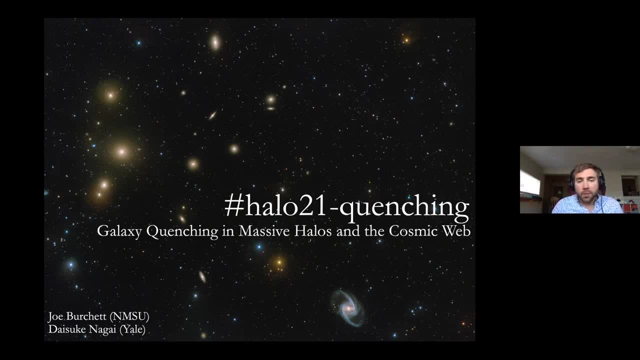 evolution. far from far from things are far from being over in terms of the impact this environment is is having on the galaxies. So you see lots of star forming galaxies in this cluster, in addition to the more red and dead population that you might find dominating more massive clusters. 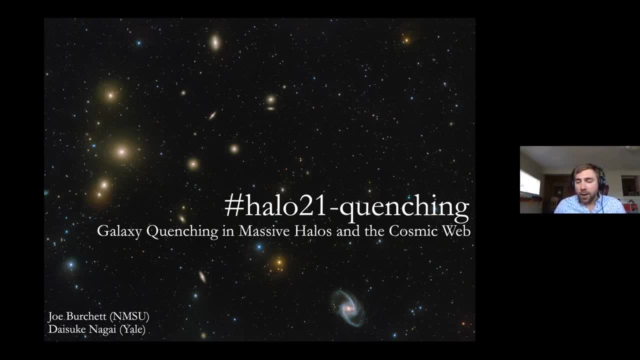 And so, however, a point that you know: I think we've sort of refined our mission statement a little bit, And I'll come back to this in a bit, but if we could refine, you know, so what we, what do we mean in in massive halos? 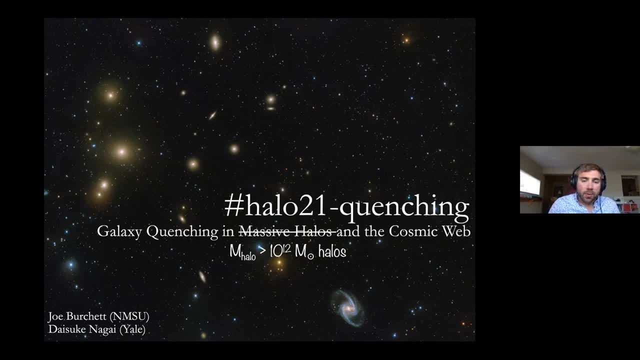 And so this is you know, I would say halo masses host halo mass ranges greater than 10 to the 12 solar masses. So this includes the environments of Milky Way type galaxies and the dwarf population in our local group, through galaxy groups and all the way to galaxy clusters. 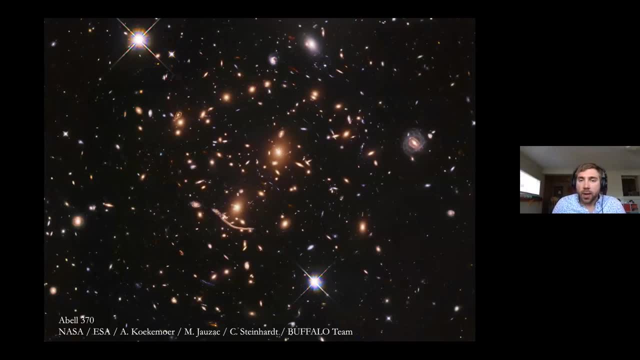 So what do gaseous halos have to do with all of this? So this is maybe, Maybe, something that looks a little bit more like the prototypical galaxy cluster being completely dominated by, by quenched, you know, red and dead galaxies. 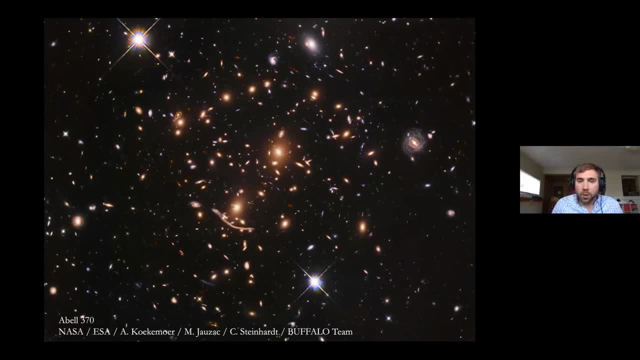 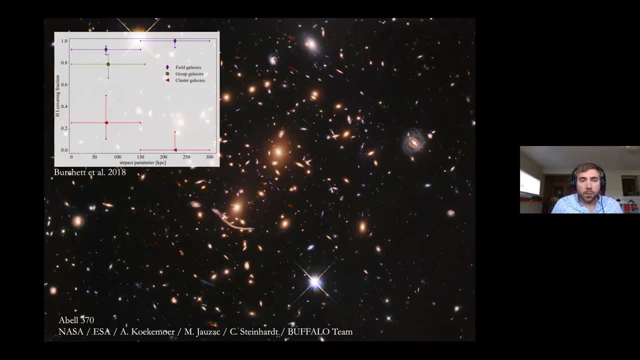 And so, really, in terms of the galaxy evolution that's going on within this environment, the circumgalactic medium very much is the point of contact, mediating environmental impacts on, on galaxies, And so I just show here: this is the H1.. 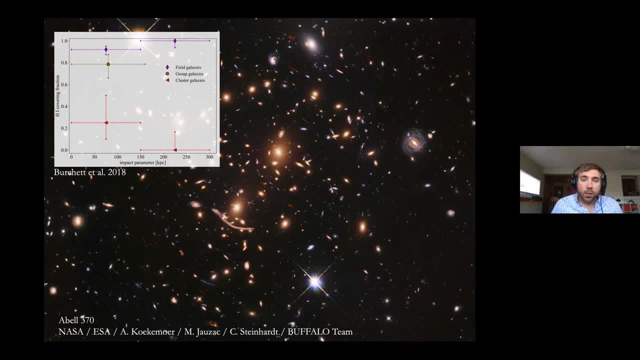 And here's what we see in this example. So we have a part of a covering fraction around the CGM of individual galaxies within various environments. So from purple to green to red, we're moving from field galaxies into group environments and then into cluster environments. 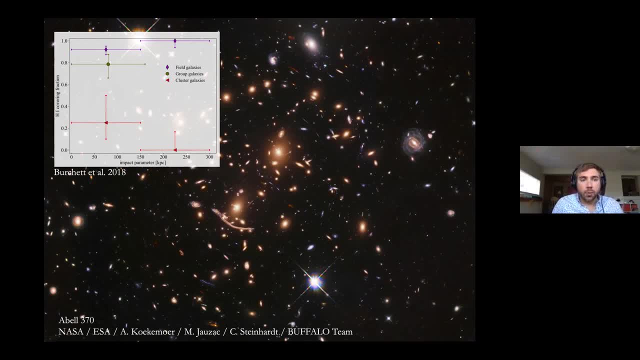 And we see a clear suppression in the CGM H1 contents of galaxies as we move into denser and denser environments. So perhaps this is an important piece of the puzzle in terms of how we can improve galaxy evolution and how we can improve galaxy evolution within the galaxy. 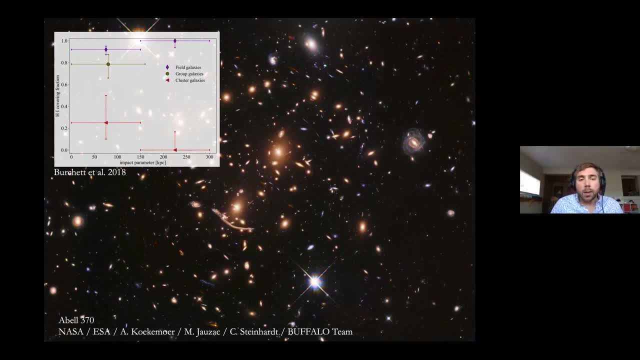 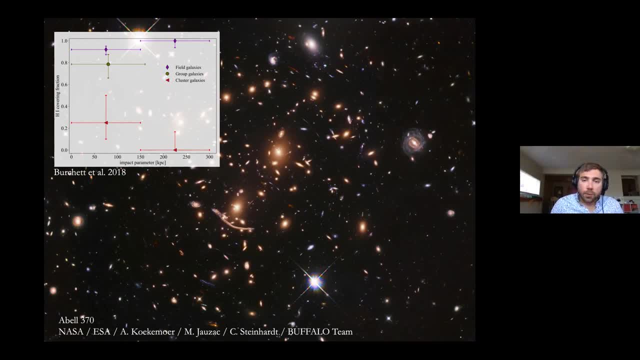 nicely illustrated that the hot atmospheres in you know, around galaxies, around galaxy clusters, so this is presumably filled with, you know, a very hot intra-cluster medium, and then you know what I'm kind of plotting here is would be the gaseous contents of halos. 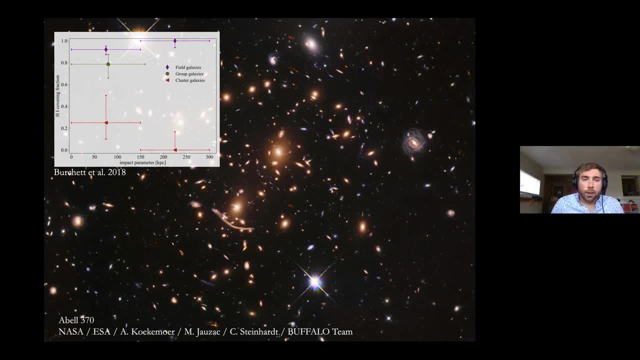 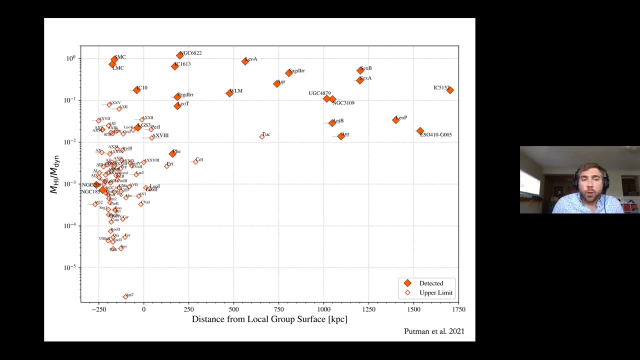 surrounding each of the galaxies within the galaxy cluster. So I think this is potentially an important mechanism that we would like to know more about, and we are sort of in early days trying to understand this relationship And really, I think what led to us refining 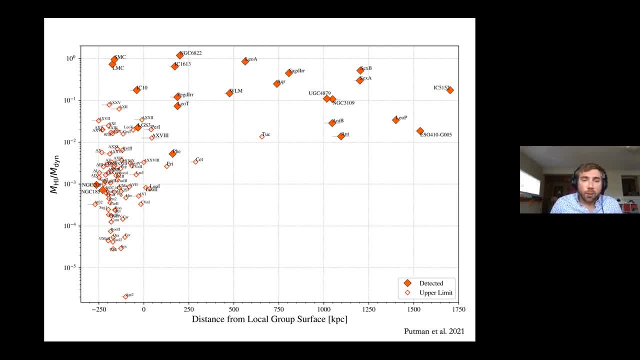 our mass regime where we want to think about environmental effects and quenching in halos comes from this work that Mary Putman showed earlier on in the workshop and also at one of our two after parties we've had. So this is showing that, as a satellite, galaxy's location within the local group is very much correlated with whether or not 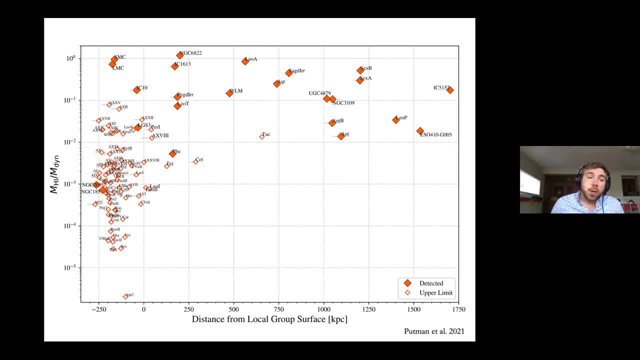 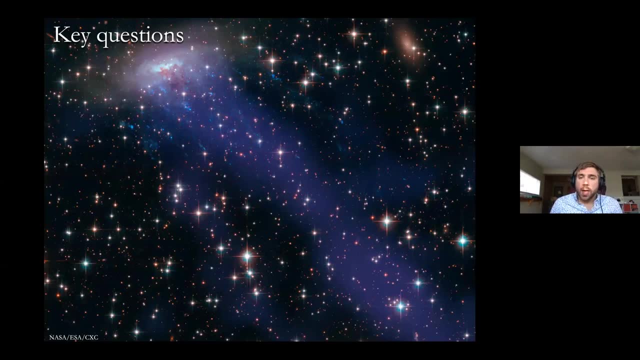 the galaxy has a gas supply remaining in it. So these are all non-detections, the open symbols here you see, at small group-centric radius for the Milky Way satellites, And so some key questions that I think we've sort of decided on and are converging on pursuing in this group. 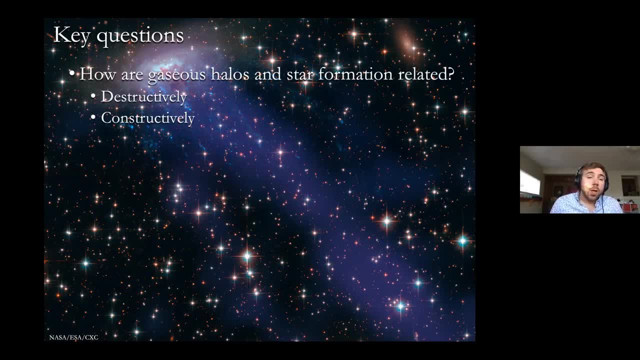 how are gaseous halos and star formation related? So I've talked about destructive mechanisms, but there may very well be some constructive mechanisms too, as seen in this beautiful jellyfish galaxy here, where we see star formation occurring in this rim pressure, stripped tail. What are the dominant quenching mechanisms? Now, this is likely to vary as a. 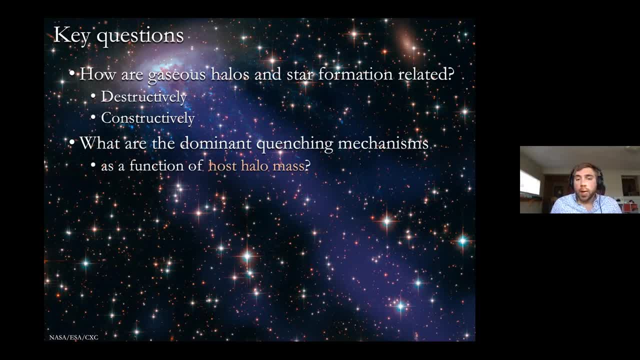 function of host halo mass. What's quenching galaxies in massive, say 10 to the 13 solar mass? halo mass galaxies might be very different than what's happening in galaxy clusters As a function of galaxy satellite mass, the more massive Milky Way dwarf satellites, for example. 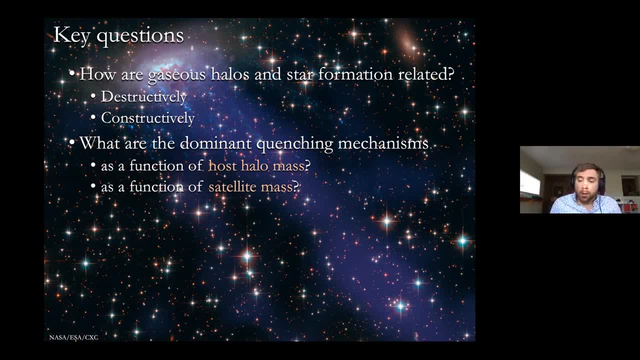 seem to be able to hold on to their gas supplies, which is presumably going to affect their ability to continue forming stars. State of satellite infall. the relationship of whether a satellite is falling into a more massive halo, for example, or whether it's on a more mature dynamical state. 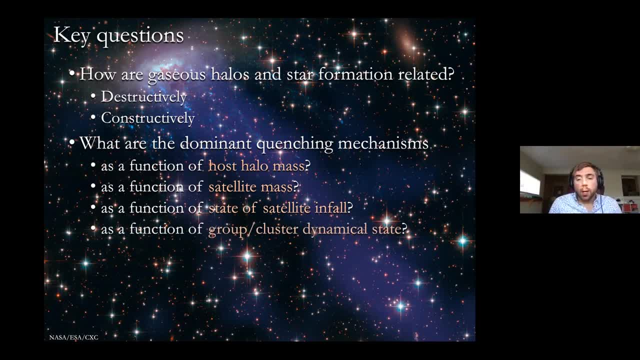 And then, lastly, the dynamical state of the group and cluster environment as a whole. We find that more dynamically relaxed environments tend to have a hotter intercluster medium, for example. So what is the role here? Perhaps a precursor to all of this? what is a quenched galaxy? 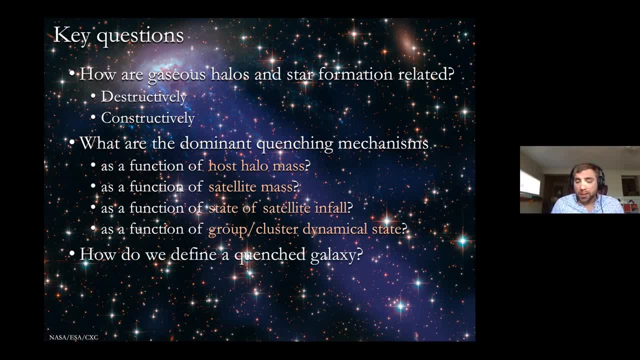 Differing definitions certainly exist. And then, lastly, what are the observational indicators of any of these points that I've raised thus far? So I think over the next week and two weeks- perhaps you know- we really like to drive towards this final point, so that we can. 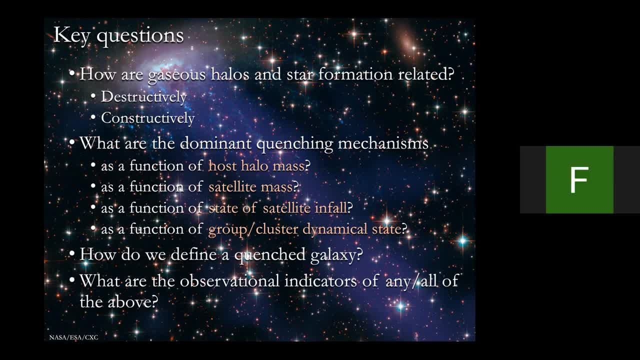 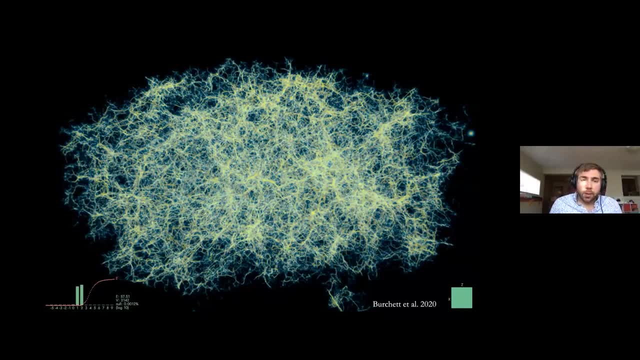 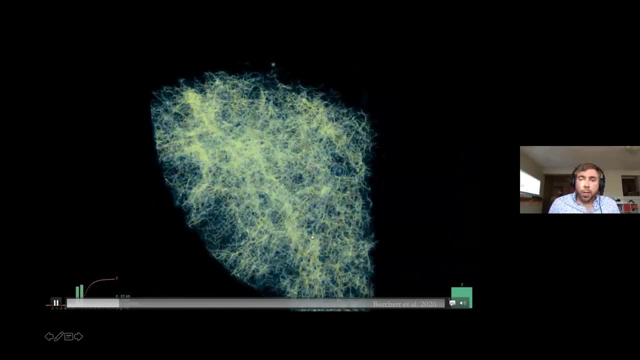 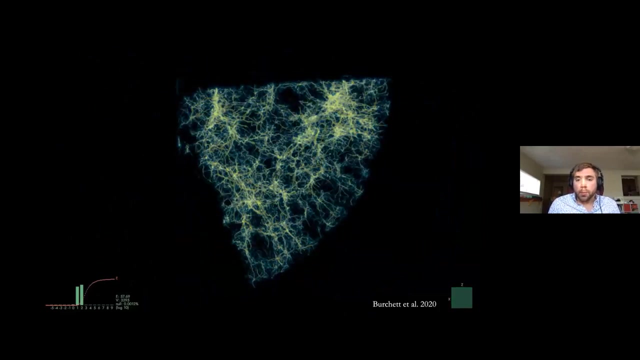 you know, make some progress in this field. So one thing we haven't yet really talked about, and I would personally like to- I'd like to hear from some of you your thoughts on this. But this is our teams cosmic web reconstruction scheme showing the large-scale structure fitted from the Sloan Digital Sky Survey. 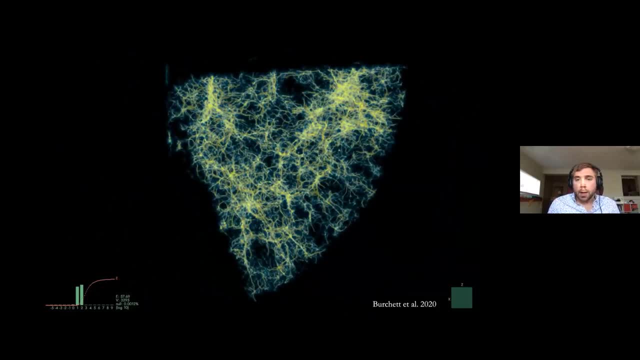 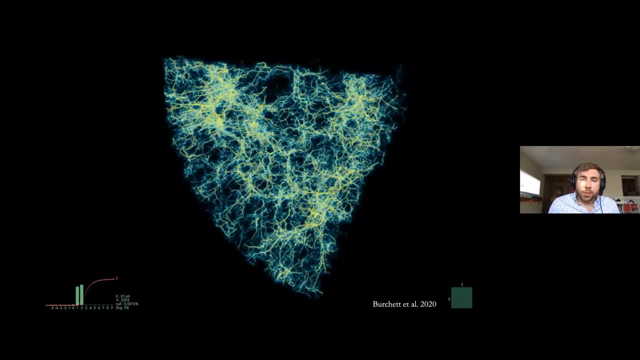 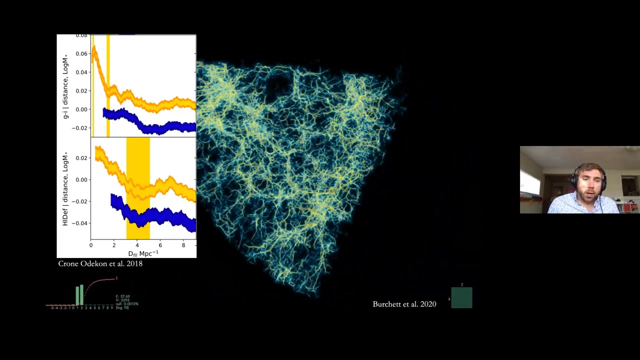 from spectroscopic galaxies out to about a redshift of 1.. So might have a little bit of a there. You know what is the impact of large scale structure on gaseous halos and therefore the galaxies that reside within. So this is just one result from Chronotocon et al of 2018, showing that, as a function of filament centric distance, galaxies tend to be redder towards the spines of filaments. 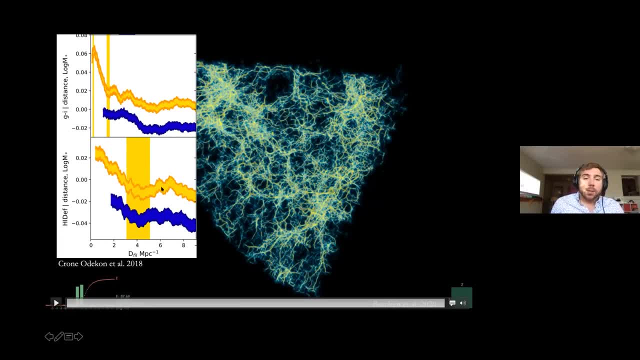 And in their H1 contents, at least in the disks of galaxies, those tend to be more H1 deficient towards the central regions of filaments. So yeah, we really haven't kind of gotten into the large scale structure aspect of this, which I hope we can. 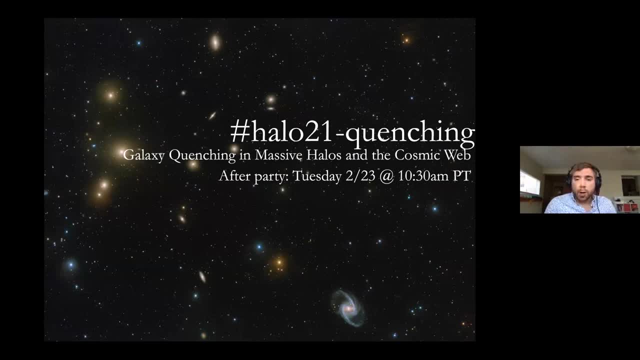 And lastly, I'll just advertise our after party tomorrow. That's Tuesday, February 23rd, at 1030 am Pacific time. So that'll be it. We'll leave about a half hour break between our keynote session tomorrow, which I'm very much looking forward to, and our Halo 21 quenching after party. 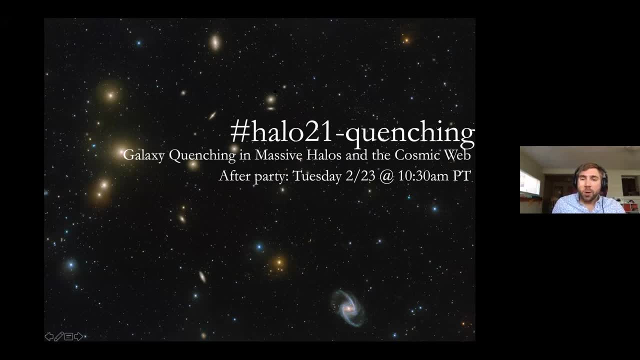 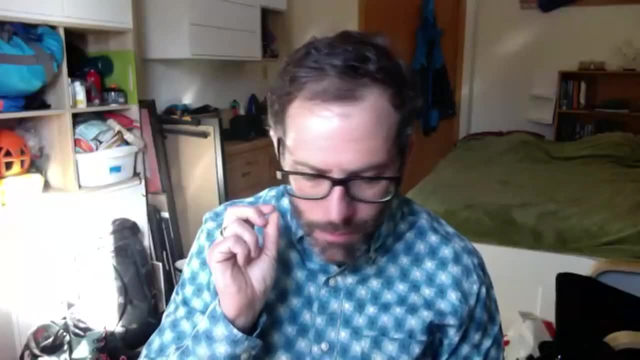 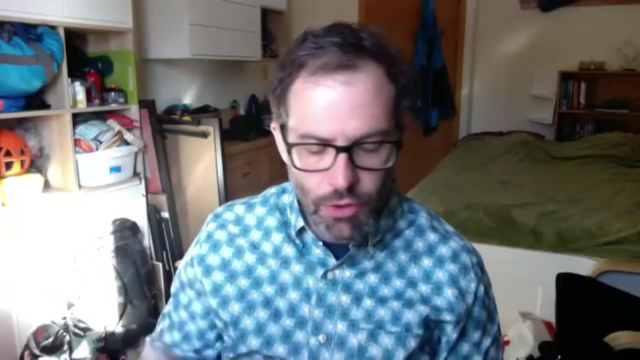 So thank you and hope to see you tomorrow. Look for a lot more updates in the Slack chat. Great, Thank you, Joe, And we will make all those announcements in the, you know, in the tutorial section, in the tutorial Slack channel. 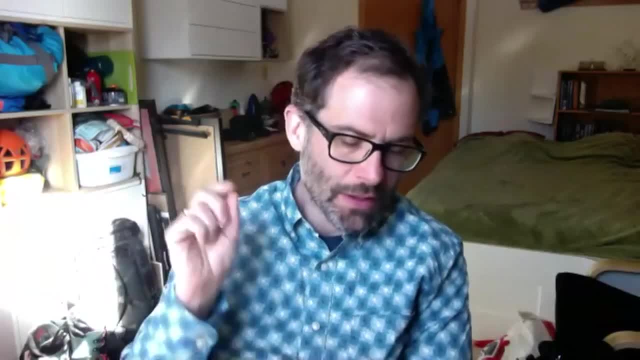 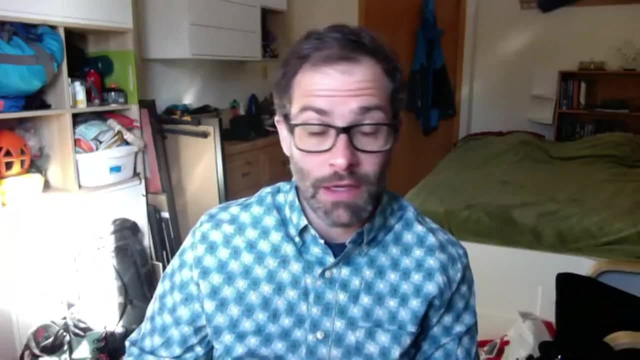 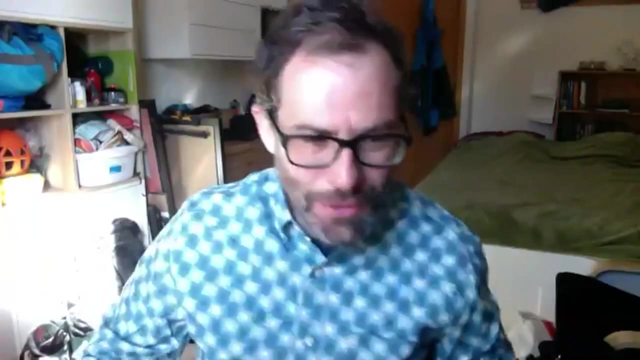 I also want to remind People that the Staircase talk today- the information, the link for that is in announcements as well as general- Looks like we will have an active day tomorrow. Two consecutive after parties: 1030 and 1130. 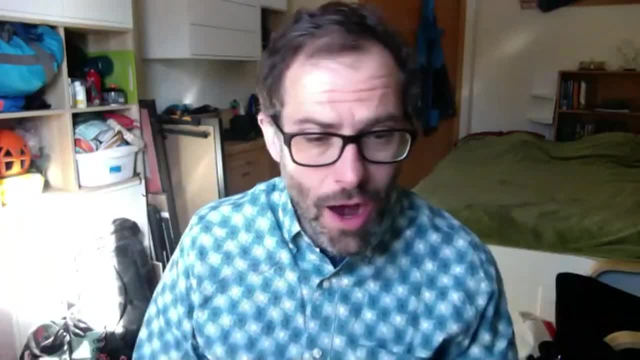 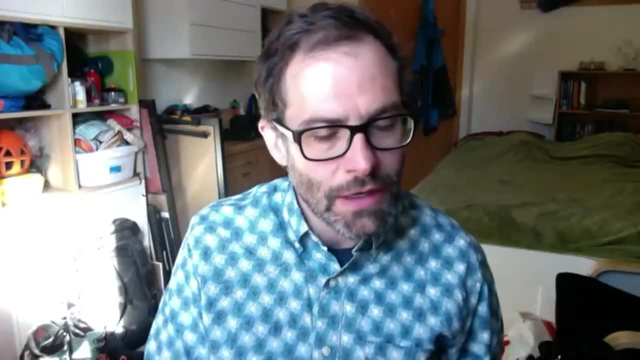 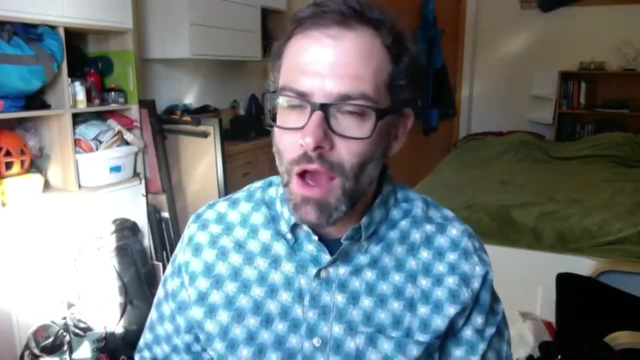 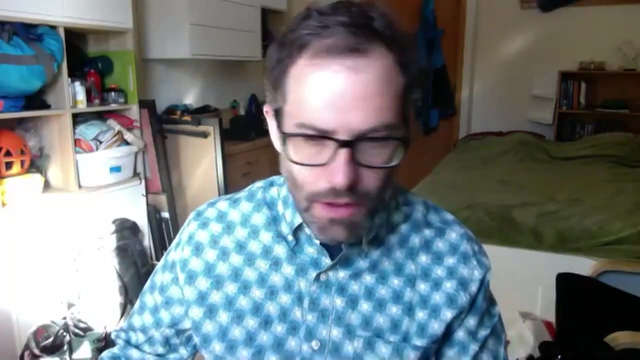 And I'm going to definitely attend both. So Mondays are for the latter half. After we do that, we'll be back After we do. the introduction of the featured conversations is: we do speed collaboration and I am going to- we're going to about about to have a coffee break here just for like five minutes, or just a quick break and then start speed collaboration. 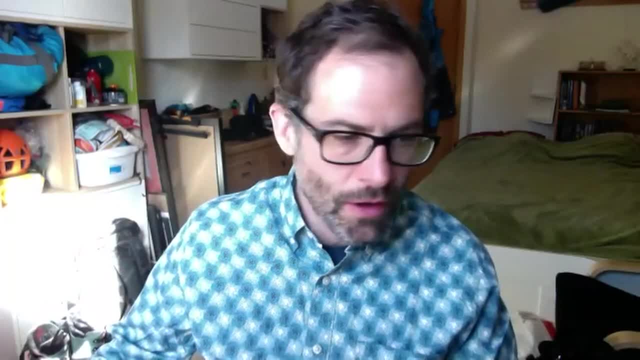 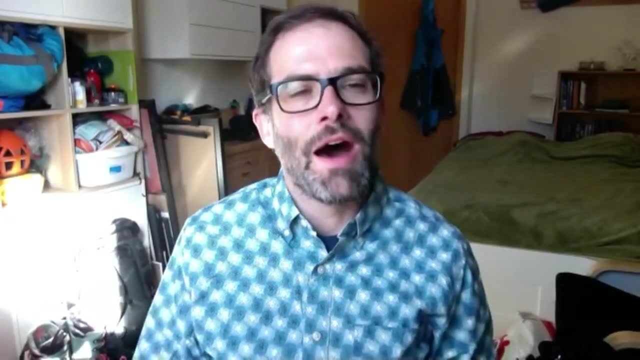 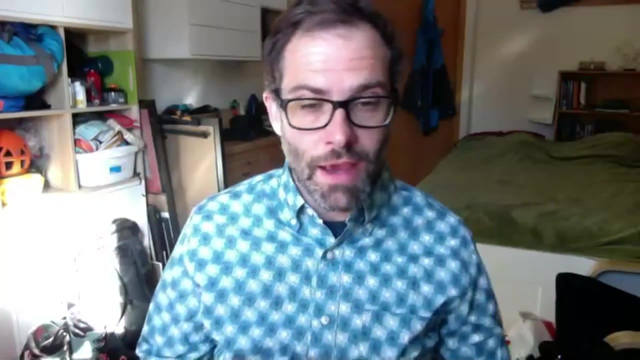 But before I do that I'm just going to share kind of the. you know the reasons why we do speed collaboration. It is to mimic. You know what we can't do in a in person conferences. It's like having an extended coffee break and mingling and talking one on one with people. 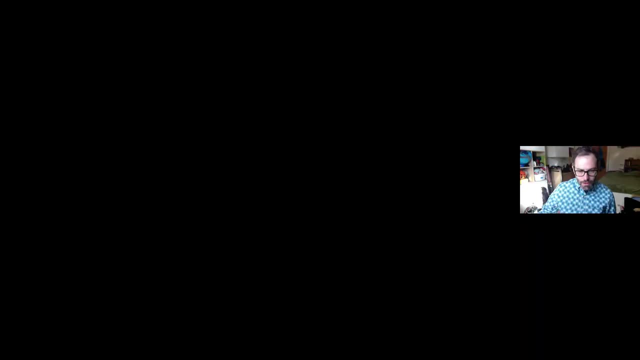 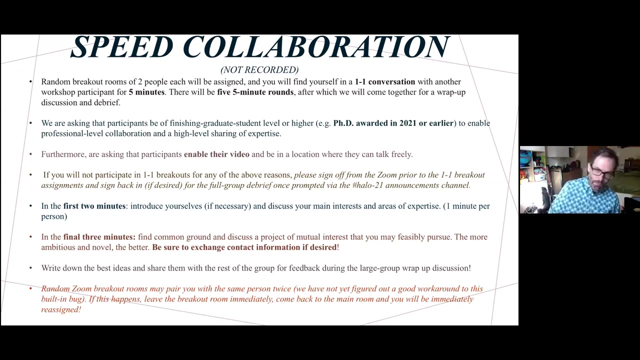 So let me share our Speed. collaborations slide And I'll just leave this up. This is for you know, we definitely want people to participate. You know, end of PhD And BE Ons and we highly recommend that you enable your video and we'll have five rounds today. 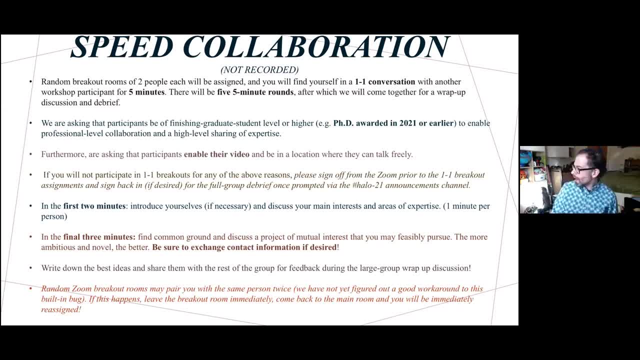 So, given that it is about eight thirty nine, let's take a little bit of a break. I'm going to get some coffee and some breakfast- I haven't eaten yet- and then be joined here at forty five after So. see you In five minutes.